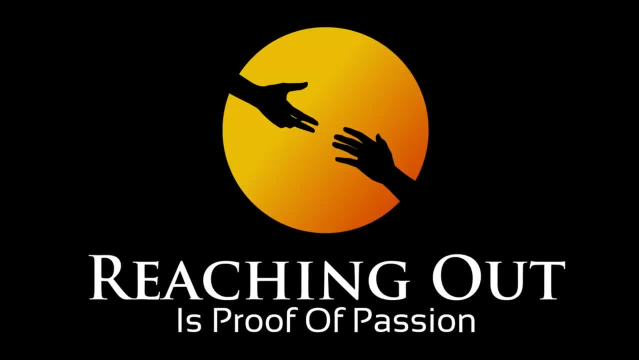 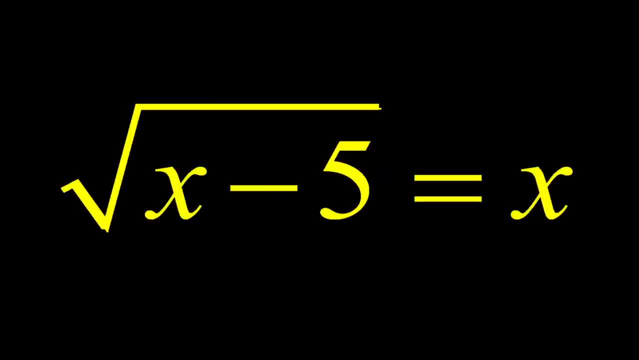 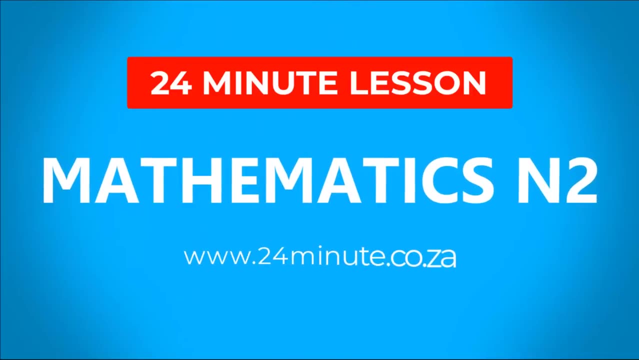 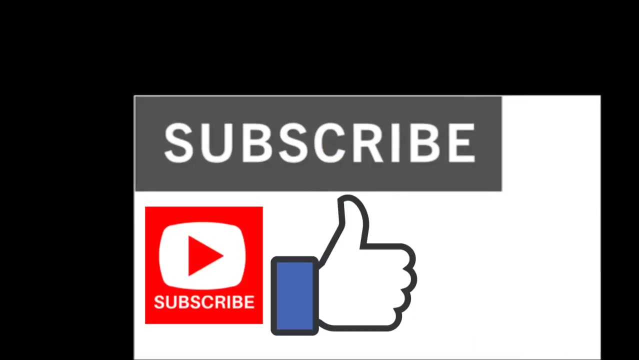 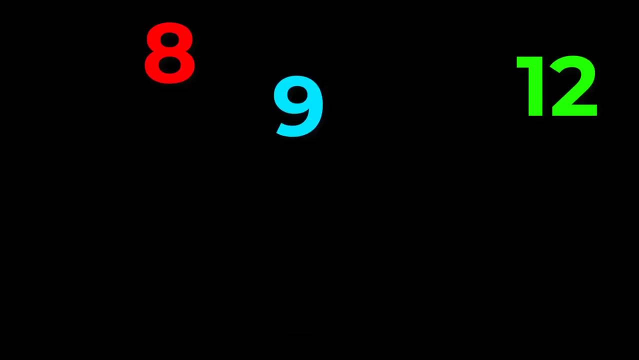 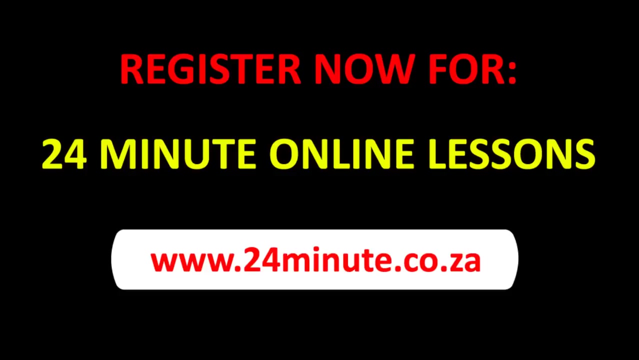 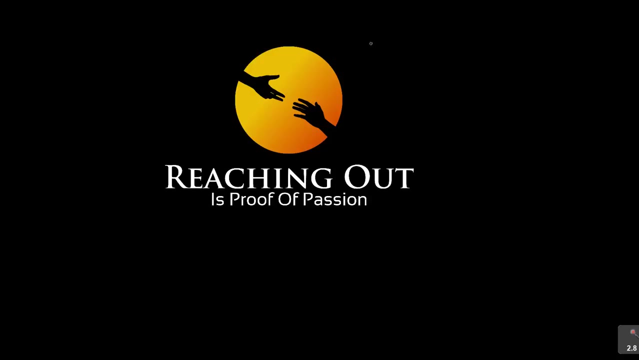 The video is not suitable for all audiences. The video is not suitable for all audiences. The video is not suitable for all audiences. Hello, our most developed student. My name is Confident. Welcome to our live session. today I thought of coming to you guys. 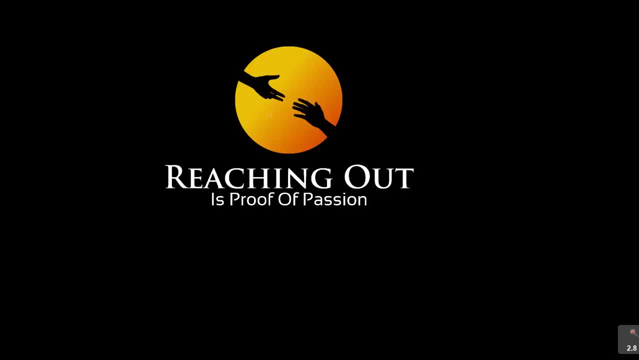 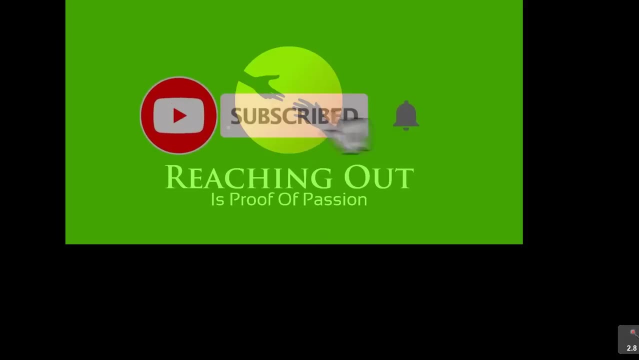 And doing some revision session, especially for those of you who are writing their mathematics. So I will be in the next coming few days. I know some of you are writing their mathematics N1, N2 and N3 in the next couple of days following. 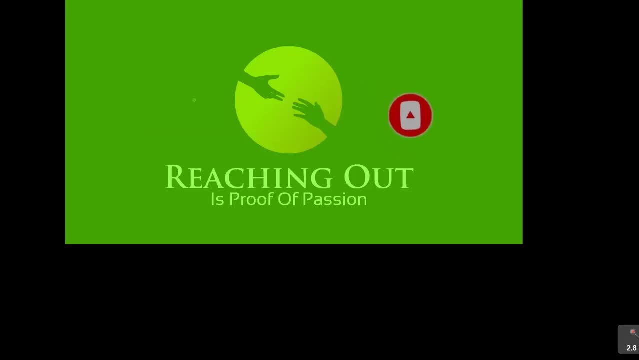 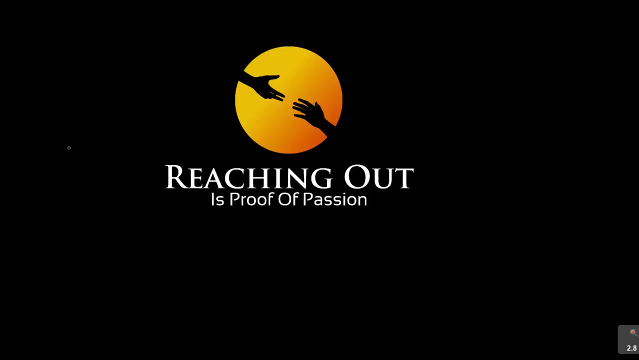 So I thought of coming to you guys and we do a quick revision, Especially when it comes to the first question, where most of you always have challenges. So this session is dedicated for those who are writing their mathematics, And today I am sharing with you mathematics N2.. 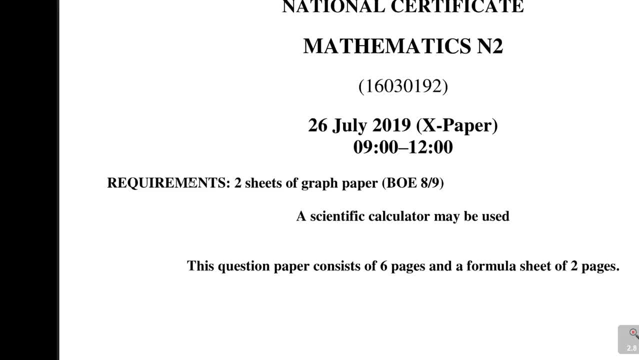 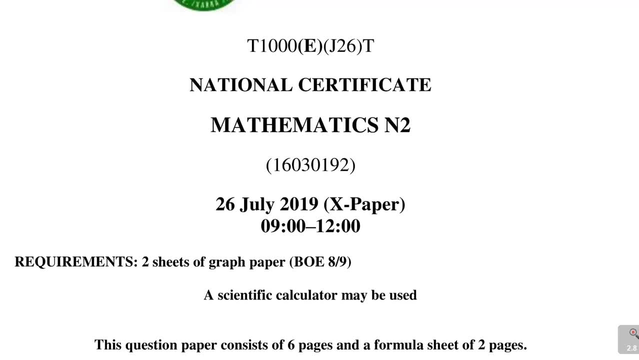 And, as you can see, I brought in a past paper, So this is a previous paper that was written. if you can see, This paper was written in 2019.. So this is June, on the 26th of July 2019.. So, as I say, mathematics N2.. 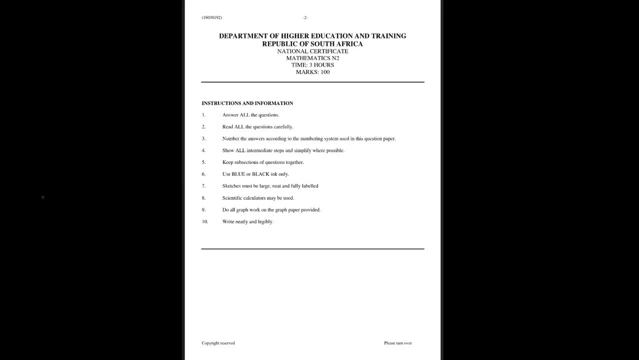 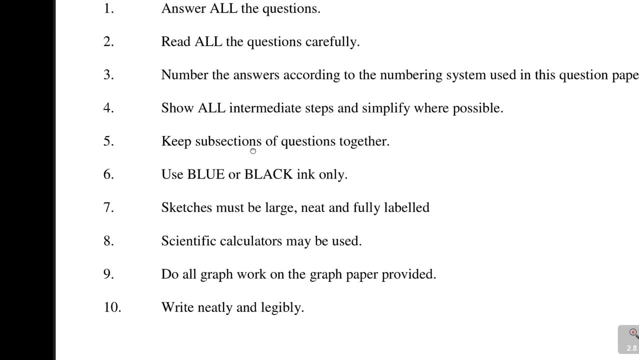 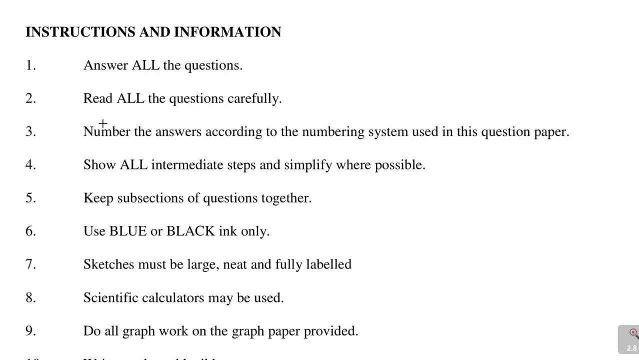 And guys, my focus here is on the first question And, of course, there are a few things that I always encourage you guys, Whenever you are going through your answering, to take note of, The first one being, if you are answering your paper, They usually here say: show all the intermediate steps and simplify where possible. 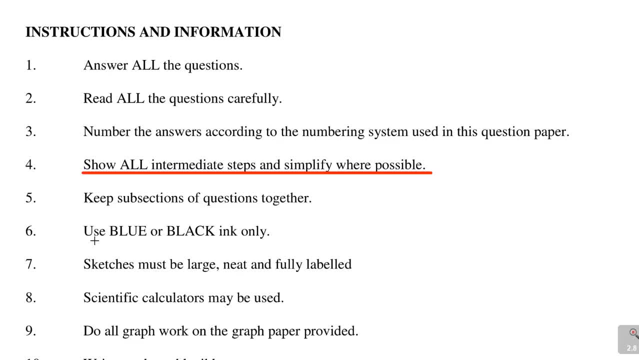 So it's very, very, very important To do that, And then, of course, you need to use the blue and black ink only, But this part is where most of the students usually leave most of their marks in their rough work. They do their rough work in the question paper. 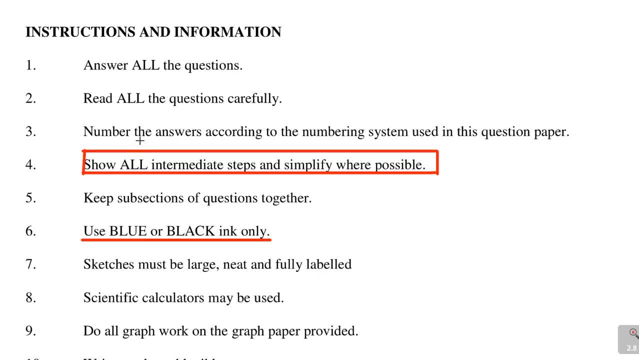 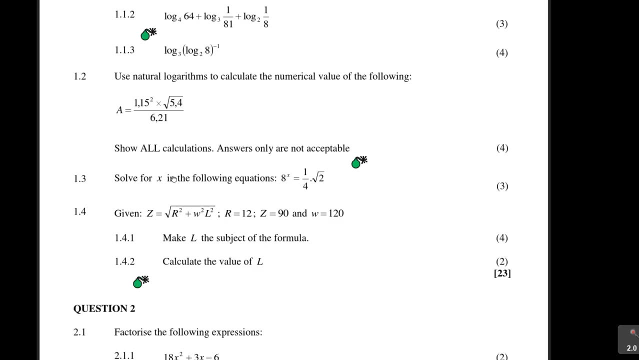 And then they don't transfer that work into the answer script. That's why it's very important for me to emphasize that the intermediate steps are very, very important. So remember that, guys. But, as I say, my focus is on question number one And I hope you guys are able to see the live streaming. 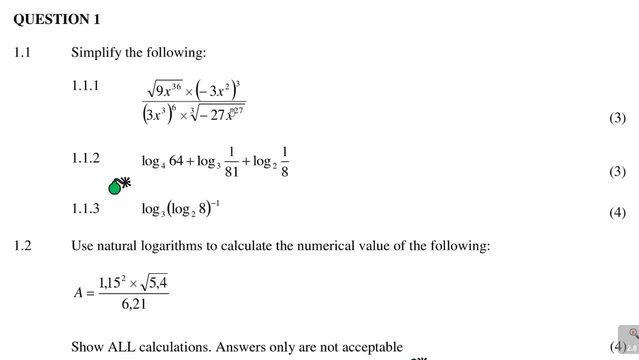 And I just want you to tune in to the next live streaming that I'll be bringing in From half past 10 in the next few coming days, Just before the exams begin. So let us look at this, question number one, And then, as I say, I just want to focus on the algebra part. 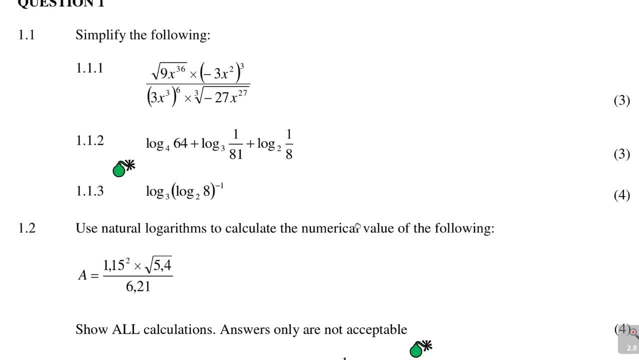 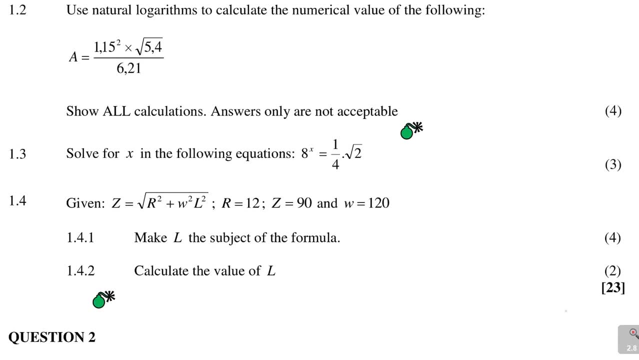 Question number one And this question. it carries good marks And you can see this is 23 marks, guys, Just think about it. And you don't want to lose 23 marks in your final exam, So you just want to maximize that. 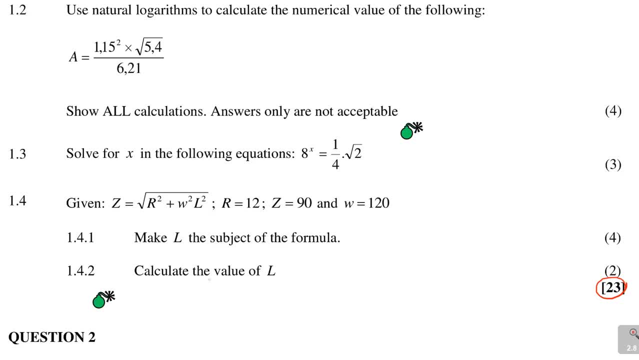 By the way, remember this paper is out of 100 marks And from these 100 marks the pass mark is 40 out of 100. So picture if you can get these 23 marks All together correct And you'll be left with 17 marks. 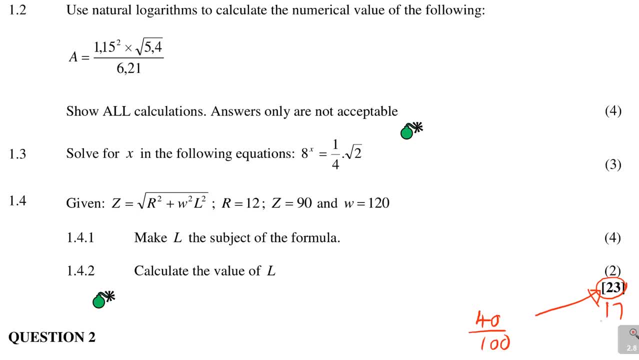 From the whole paper, you are just left with 17 marks to get a minimum of 40. So just think about it and see that this section of algebra carries good marks. Not only is it on question number one, It actually continues to question number two. 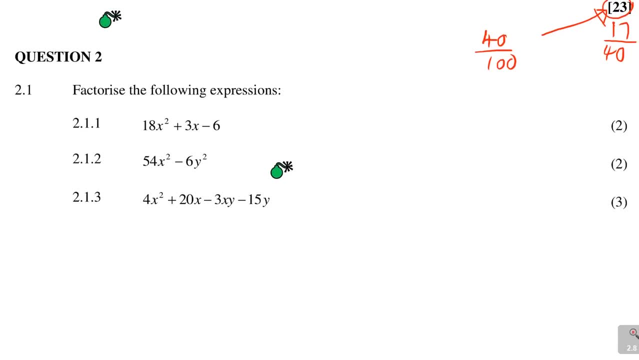 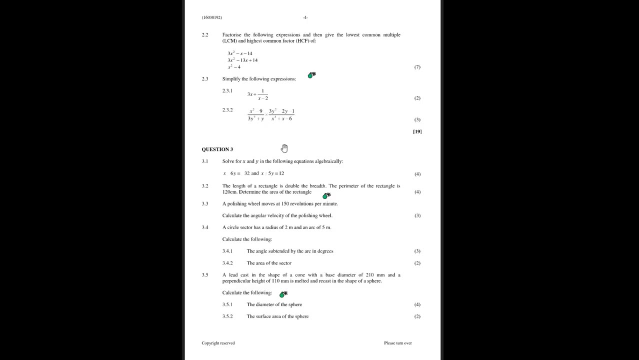 So if you can do it well again in question number two- And let me see the total mark allocation of question number two is 19 marks. So if you do question number two, Question number one, Question number two: Automatically you have passed your exam. 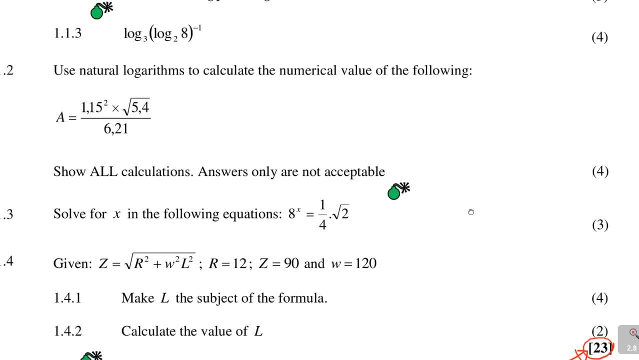 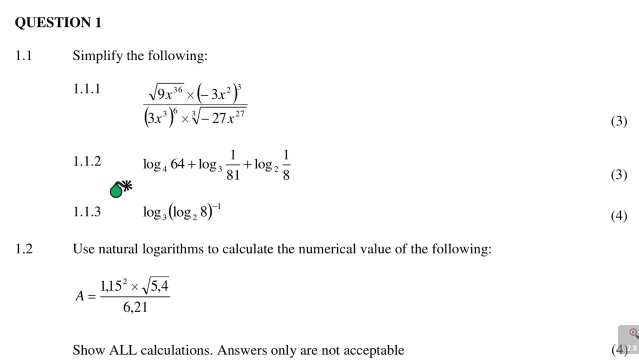 So it is very important for you to understand your algebra. Okay, having said that, Quickly, let us look at this question. I'm just going to be brief in some of the sections And I will encourage you to always go through our videos on YouTube. 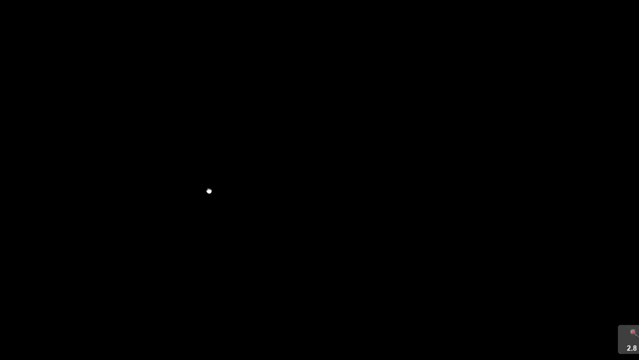 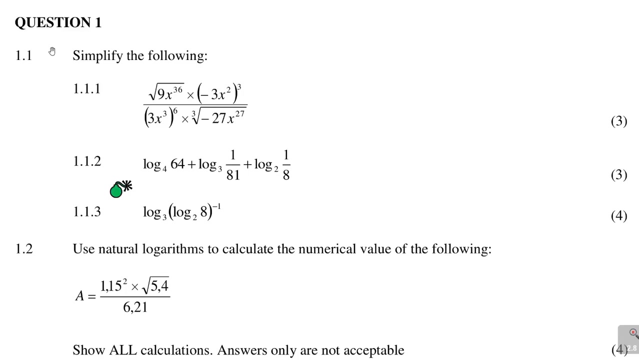 Guys, if you have not subscribed to our channel, It is a good chance for you to subscribe So that you can actually be able to take advantage of these live sessions that I'm also bringing. And on top of that, there are some videos, Lots of videos, that I have posted. 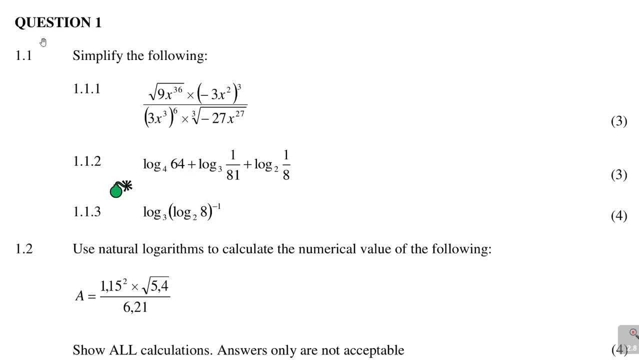 But unfortunately, if you are not a premium member, You are not able to watch those videos Because it is for those who are the premium members. And what are the premium members? Those are the guys who have subscribed. You can see a certain video says it cannot be watched by everyone. 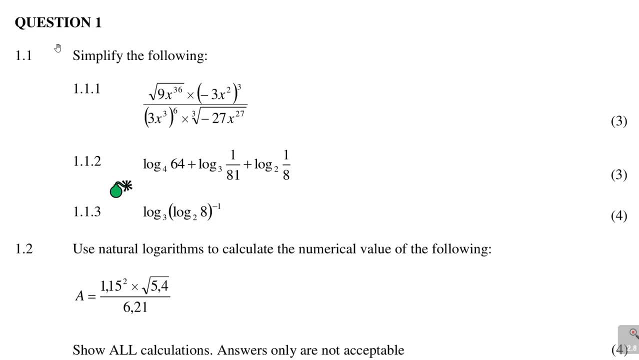 But only for the premium members. So for you to become a premium member, you just need to subscribe And there is a small fee that you need to pay monthly. You can cancel it anytime without any obligation. So if you feel like you are enough. 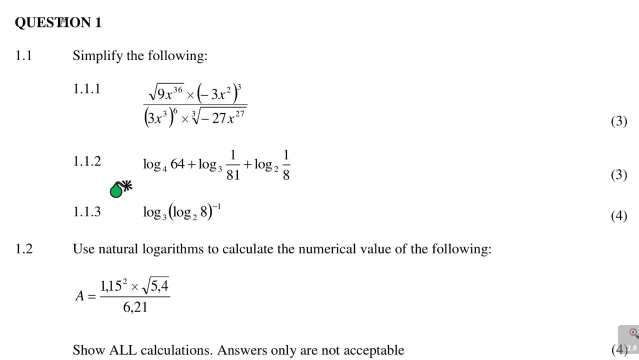 Maybe you have already written your exam And you are no longer using these videos. You can just unsubscribe from the premium membership And it starts from around 39 rand or so a month from N1.. But the main purpose of those premium members is to support the channel. 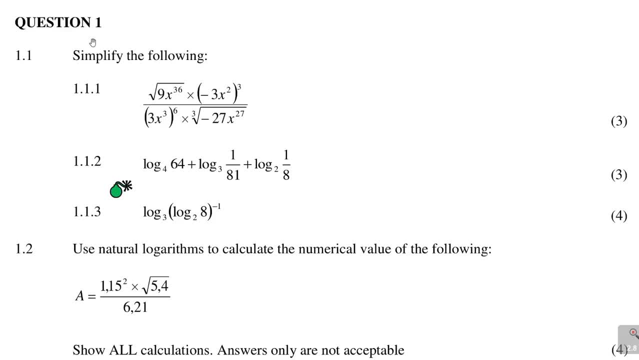 For example, If you need to bring these live videos, There is a lot of resources I have to bring in Concerning the live streaming, The equipment that has to be used, The data part of it, That you need some quality data for you to see. 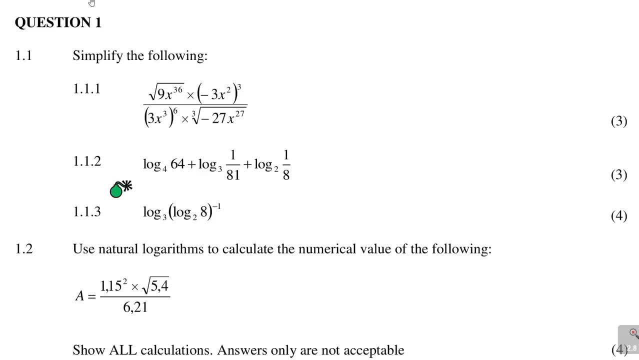 This kind of video So that there is no buffering or videos kind of tessellating. You know all those kind of problems Whenever you have got a problem with network. So such guys are helping to sponsor, in a way, this channel. If you are benefiting from these channels, 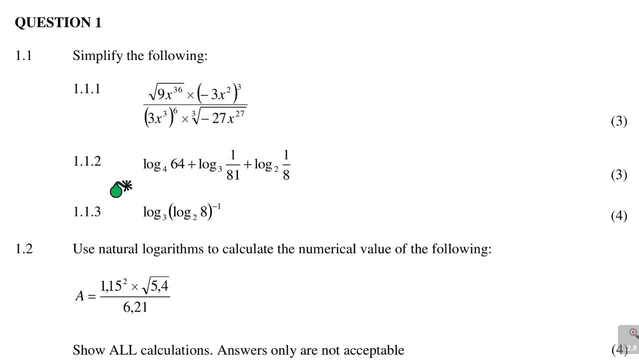 I would encourage you to actually consider joining premium membership. Now let us look at this question. It says: simplify the following And in this particular scenario, Let me try to work it from here, Because already I got good space. Now, whenever you are dealing with such a question, 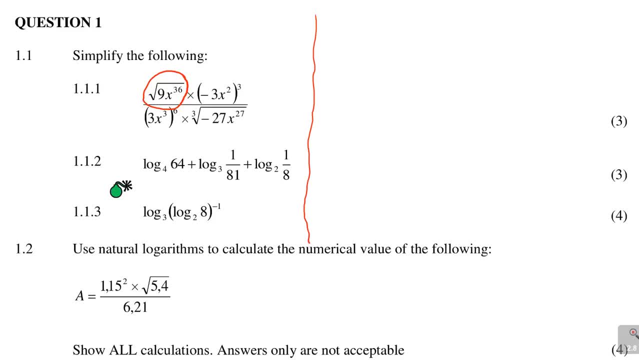 Look at this part. There is the first one. You are given to say you want to simplify that, 9x to the power 36.. In a square root Now, this square root symbol means you put a bracket And it is to the power a half. 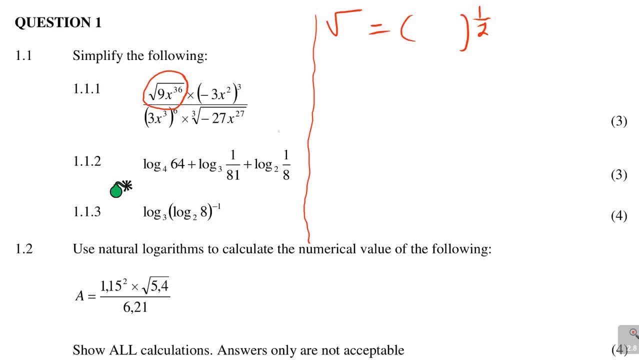 That is what this square root actually means. So you put a square root And it is to the power a half, And when you are now writing this part to say, Square root of 9x to the power 36.. What this symbol means is: 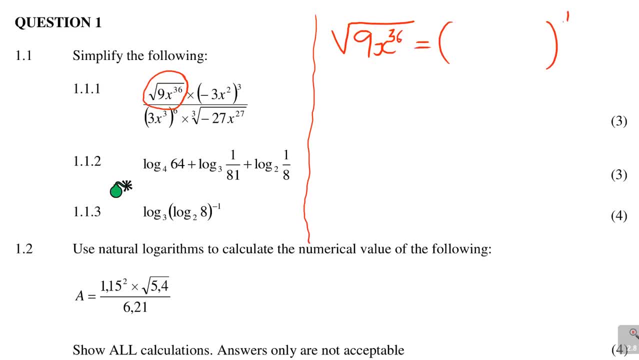 You put that bracket And then the power To the square root symbol means power half. So now again, what does 9 mean? Remember, these are exponents. You have to be using the laws. So 9 is same as 3 squared. 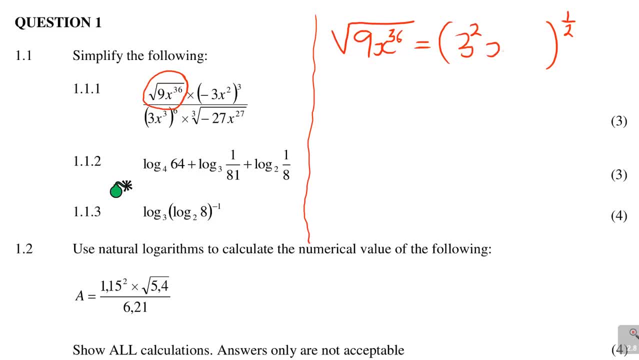 So that you can be able to simplify. Then it will be 3 squared x to the power of 36.. That is what this actually means. Now, this power half, It multiplies that And it multiplies, So the power multiplies the power. 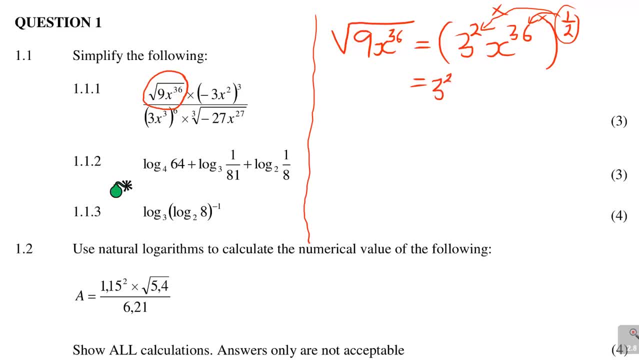 So this will symbol become like: 3 to the power 2 times a half, x to the power 36 times a half. You see what it means. And then when you have done that, The half cancels. there You have got 3x. 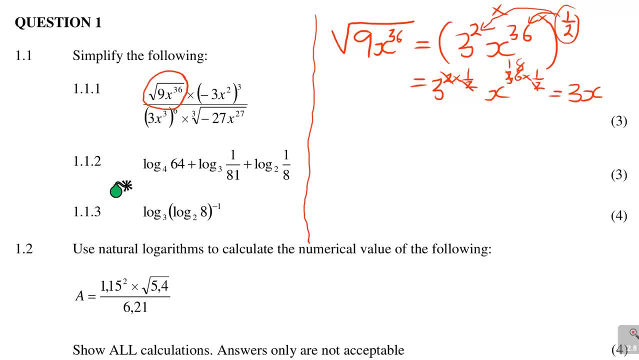 Now the half of 36. I think it is 18.. So it is x to the power of 18.. So that is what this symbolifies. So this will become 3x to the power of 18.. So you see how. 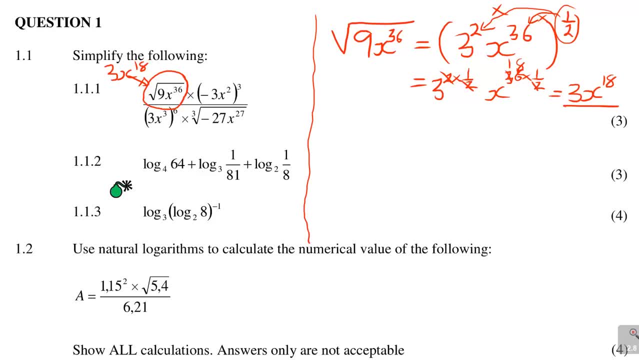 Simple. sometimes this becomes. It is just a matter of you Being able to Simplify them in a way. Alright, having done that, Let me write it down here. To say the top part there is 3x to the power of 18.. 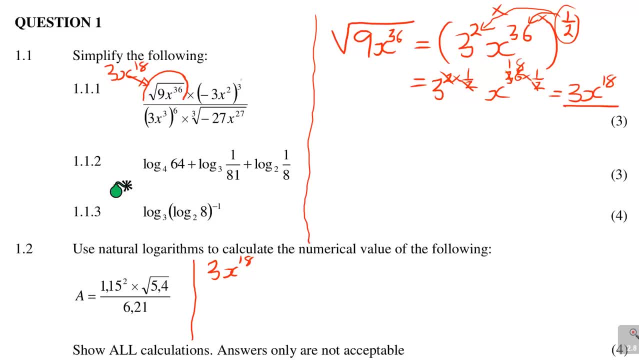 Let's move on. If I am simplifying This particular part now, This is negative 3. x squared. But there is a bracket here. This is negative 3. So this is negative 3. x squared. So how does this simplify? 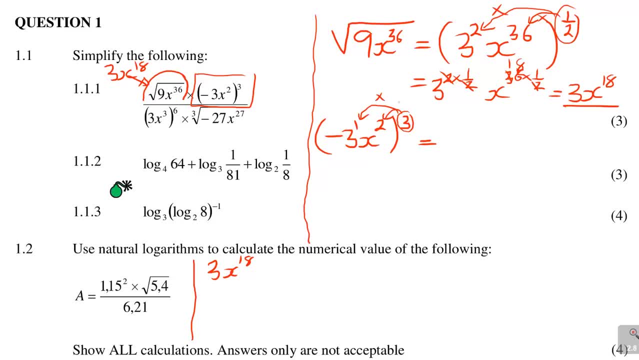 Remember, if you are not given a power there, It means the power half. So the same thing, This particular exponent will multiply that And it multiplies that. So it will be, in a way, What you are having is: Now you need to be very careful. 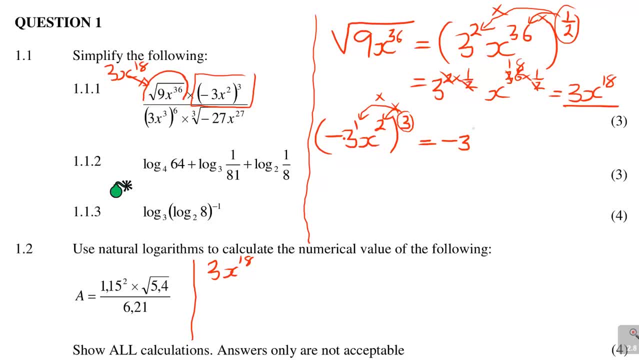 Of this negative part, Because it is negative 3.. 1 times 3.. But now Because the negative here Is not affecting the power, So it is like you have got Negative 1 dot. So you understand. So you don't need to put a bracket in that. 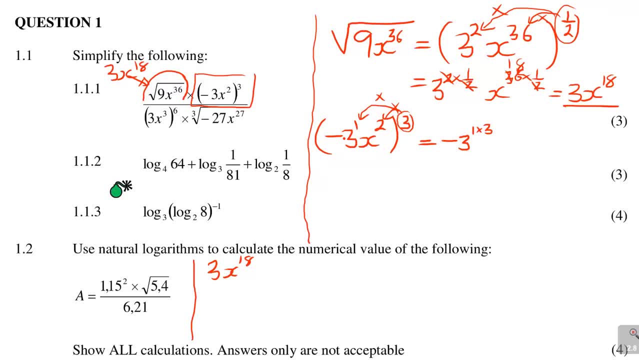 So you can just leave it like that. So what you will be having? You will be having negative 3.. 1 times 3x To the power, 2 times 3.. When you simplify that, It is negative 3.. 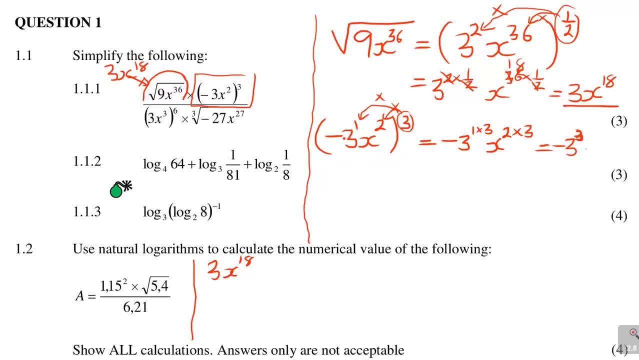 And then x to the power, 2 times 3. Is 6.. So that is that. So you will have In this scenario here, A multiplied by Negative 3 to the power of 3.. x to the power of 6.. 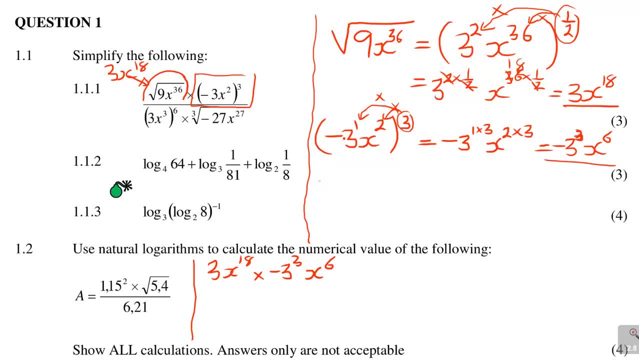 So you see that, guys, And then at the bottom, Which is the denominator, We are having that part Which is 3.. x to the power of 3. Similar to the one I just did, And then this is to the power of 6.. 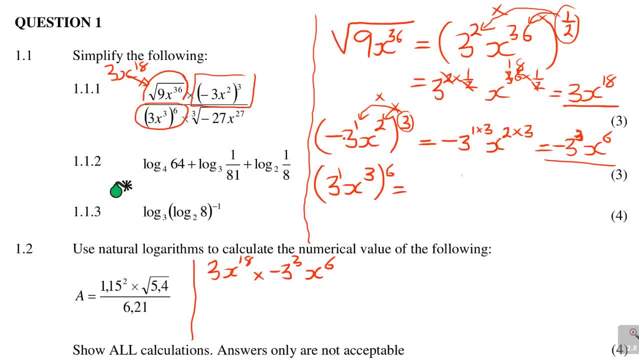 Again, you have got a power there. Whenever you see brackets, It means first you have to deal with brackets. So here is: 3 to the power 1 times 6.. x to the power: 3 times 6.. Are you seeing that? 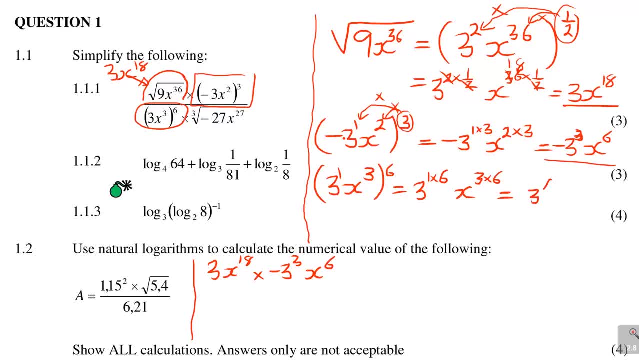 And then this is same as 3 to the power 6.. x to the power 6 times 3. Is 18.. So this is all over: 3 to the power of 6.. x to the power of 18.. 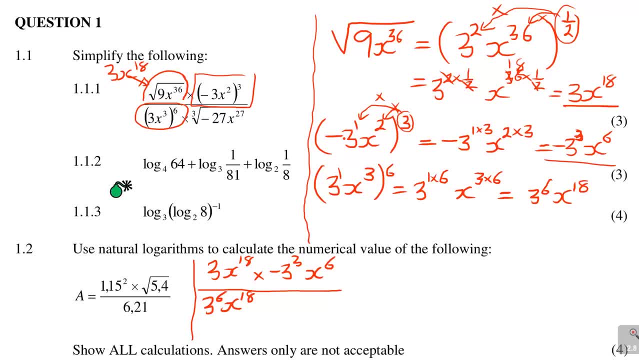 And then the last one, Which also Needs some emphasis, If I can just Create more space again. Look at this other one here. I am given this part as Alright. When you are given here a cube root, Cube root, you must know that. 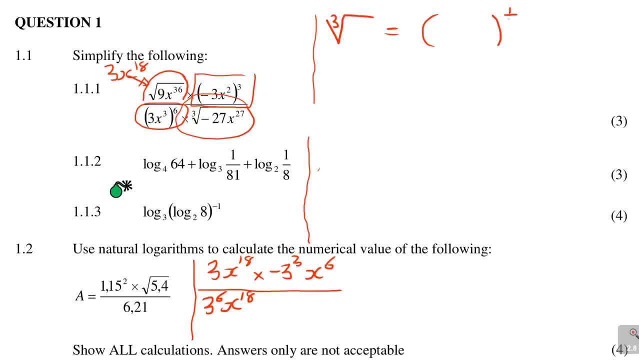 It means bracket And then it means 1 over 3.. Remember, I said, Square root means bracket And it is 1 over 2.. So if I put An a root, It means bracket And it means 1 over a. 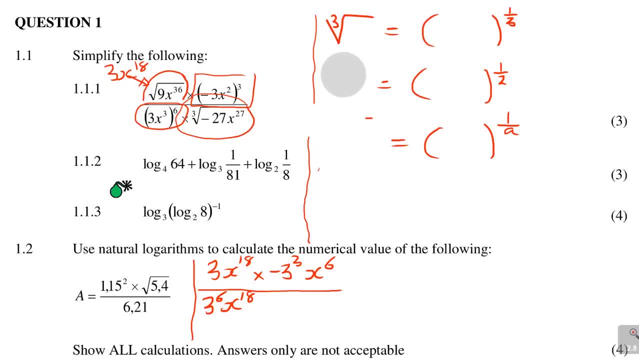 Always remember that That is what the root means. So the cube root Will automatically mean 1 over 3.. So if I am given here a cube root Of negative 27.. x to the power 27. See that. 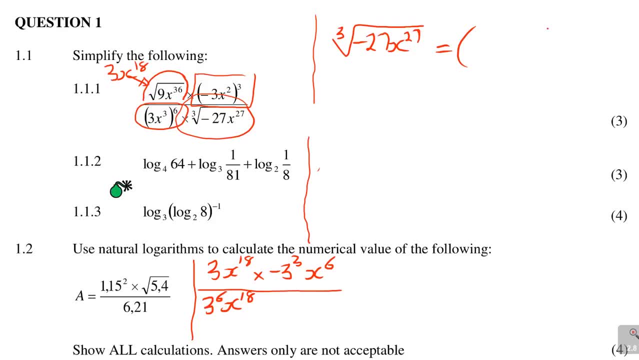 So what I have here Is put a bracket And then have 1 over 3. And then you have got now 27, remember? If you take a calculator and quickly check, Ask yourself what is 27.. 27 is 3 to the power of 3.. 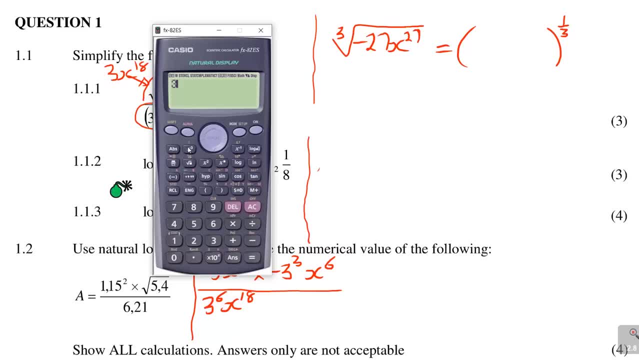 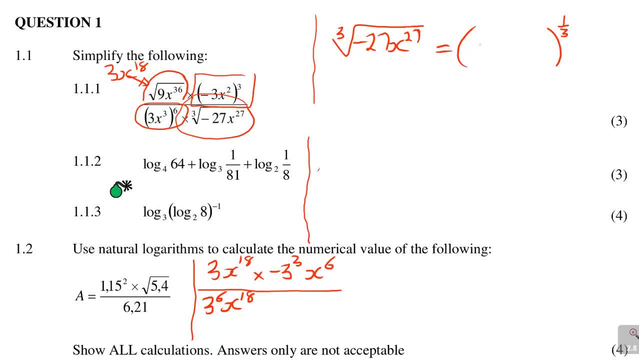 If you just remind yourself, Is 3 to the power of 3. It will give you 27.. So they always give you these numbers that are easier Or that can be expressed Either as a square root or a cube root. So it is minus 3.. 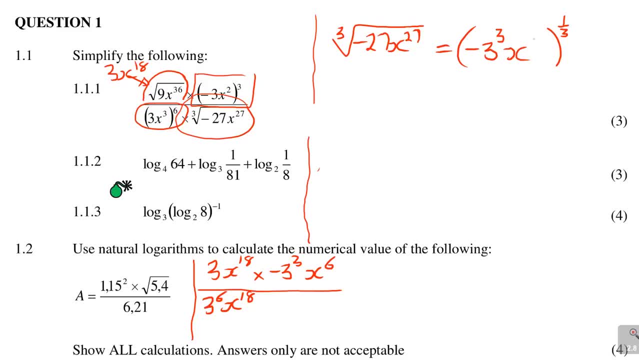 To the power of 3.. x to the power of 27.. Remember what I said: This power, It multiplies And it multiplies. You need to do this step by step, Don't just be in a hurry to try to simplify things at once. 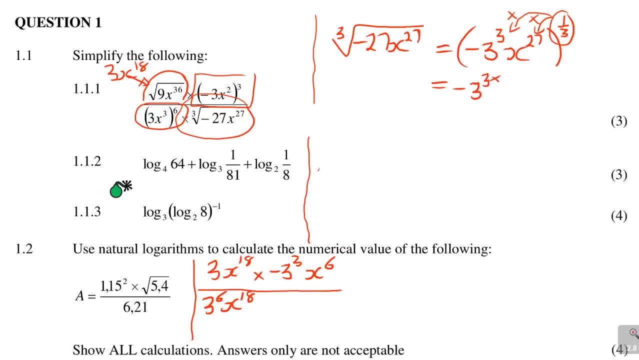 You usually make some errors. So it is 3 times Power 1 over 3.. x to the power 27. Times To the power, 1 over 3. So when you do that, It will then 3.. 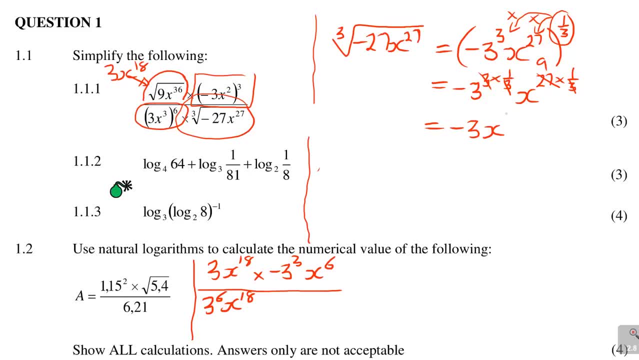 x, Now 3 into 27 is a 9. So x to the power of 9.. So that will be here to say Times Negative: 3. x to the power of 9.. So you see how this has been simplified too. 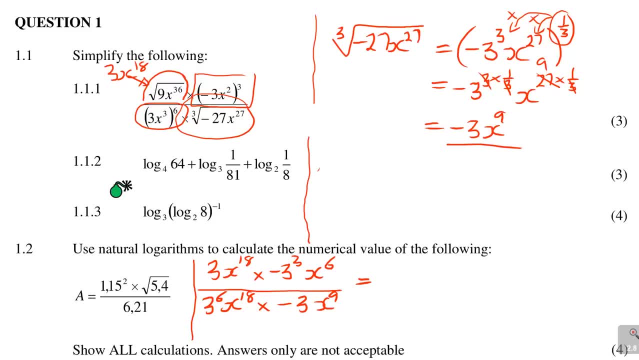 Now again Going forward. These are laws of exponents. Now, remember we have a law of exponents, The common law that is being used here, The common law that says: If you are given a to the power of m, Times a to the power of n. 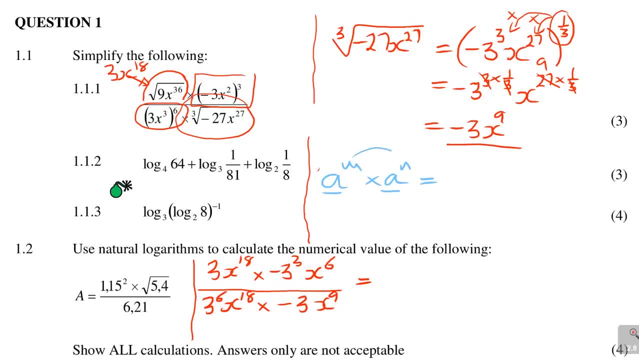 Now, when you see the basis being the same, It means you add these two exponents, You add them, So this becomes a. Then you say m plus n- Remember this law. And then we have the division part of it That I am going to apply. 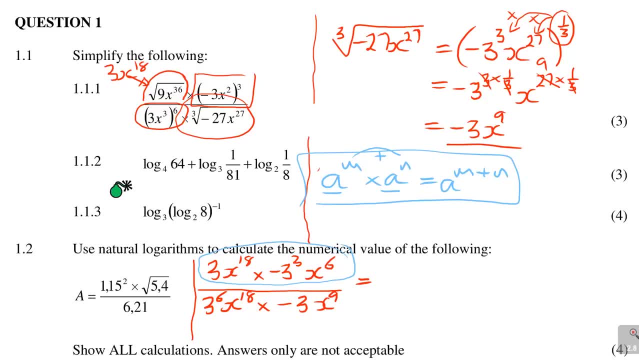 But for now I just want to apply the law at the top And I want to apply the same law at the bottom In the denominator, So let's apply it First. let's focus on 3. And 3. In this case, 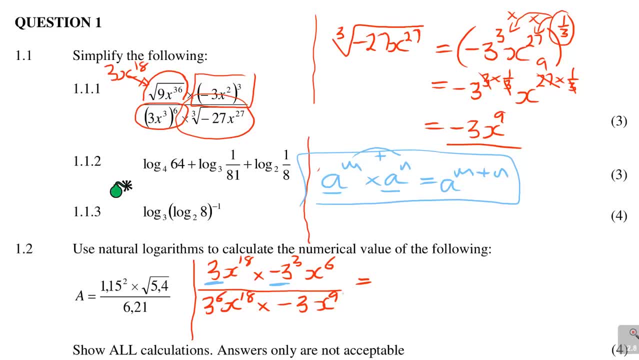 So in here What I have. I am going to write to say I have got 3 to the power of 1.. Times negative 3 to the power of 3.. And then times x to the power of 18.. 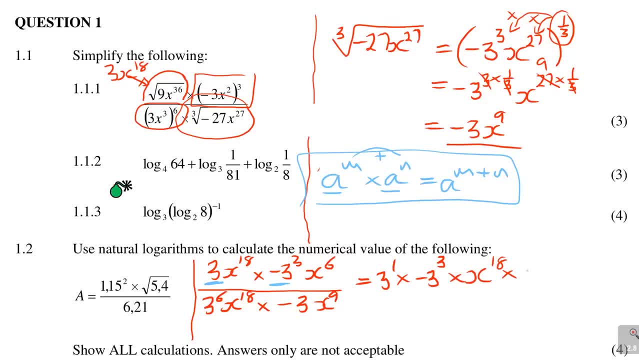 See, I am just regrouping Or rearranging this Times x to the power of 6. See what I am doing All over. And then I have got 3 to the power of 6.. Times negative 3.. 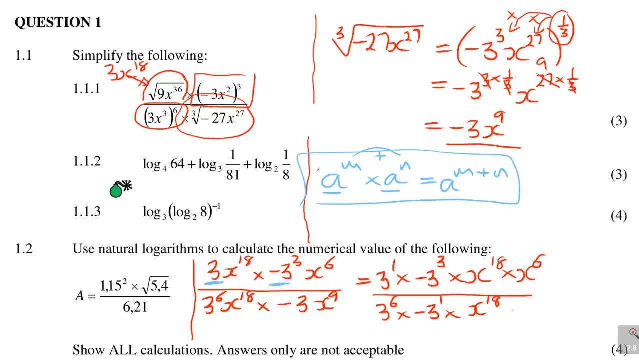 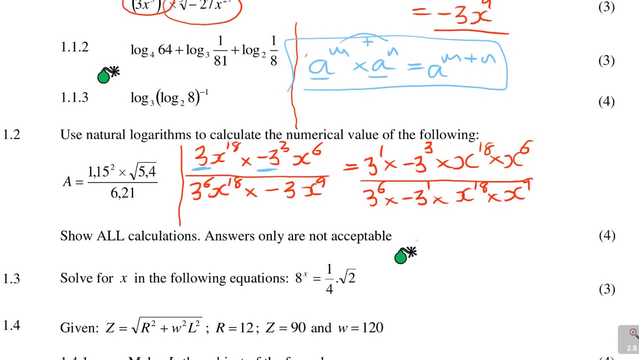 If you just see negative 3. It means there is a hidden 1. Times x to the power of 18.. Times x to the power of 9. So, Alright, So actually, That is that, This is to say. 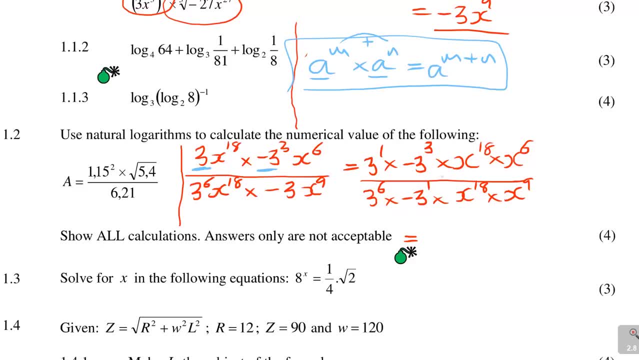 It is up to you How you would have done that, But I actually see some different Ways even of approaching this. For example, You can see that in here I have got x to the power of 18. Look at this. 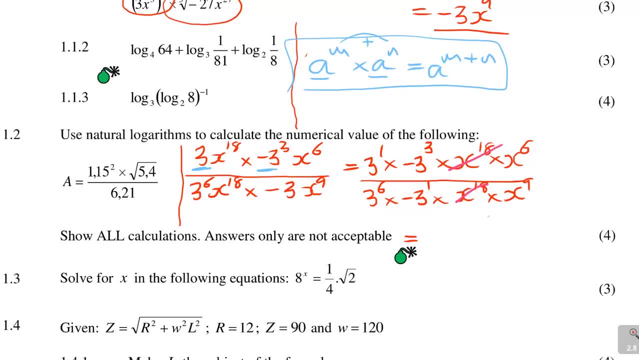 This. you can actually take it out Because it is similar. And then also The negative sign. Look at the negative sign. I have got a negative on top. I think you can see that. So now, When I can apply, then 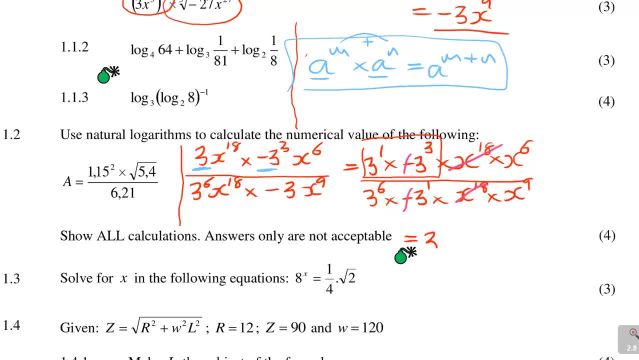 The law that I was telling you about here To say this is: See, the base is 3.. So it is 1 plus 3. Because I have to add this to The exponent And then it is x to the power of what. 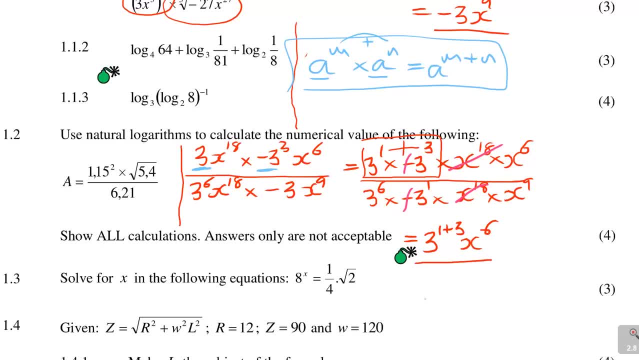 Of 6. Over. I do the same thing at the bottom: 3 to the power of 6. Plus 1. To the power of 9.. I am getting that. So 1 plus 3. Is 3 to the power of 4.. 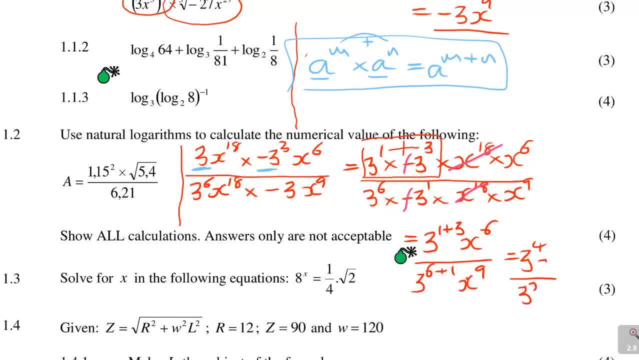 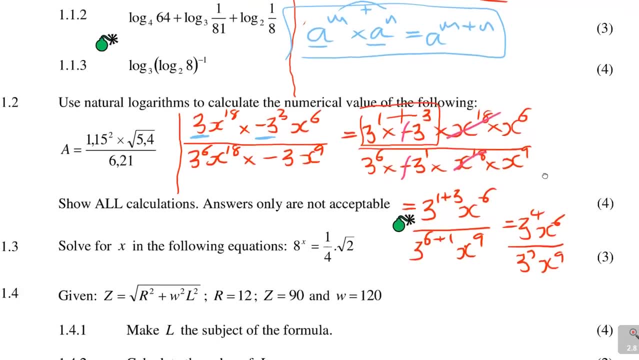 Over 3 to the power of 6 plus 1. It is 7.. But there is x to the power of 6. And there is x to the power of 9.. Now the next part Is for me to apply the second law. 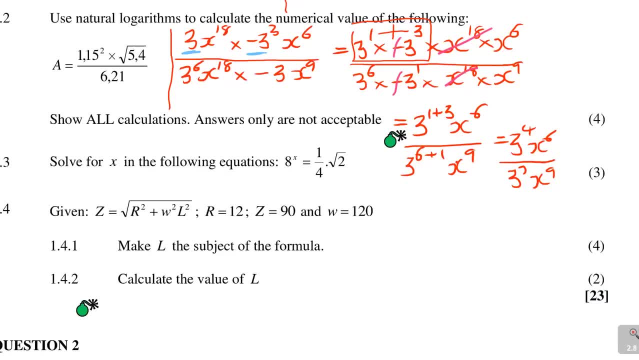 Let me just take this off Now. the second rule, Or the law says: If you are given 3 to the power of m, Divided by a to the power of n, Is equal to a to the power of m minus n. 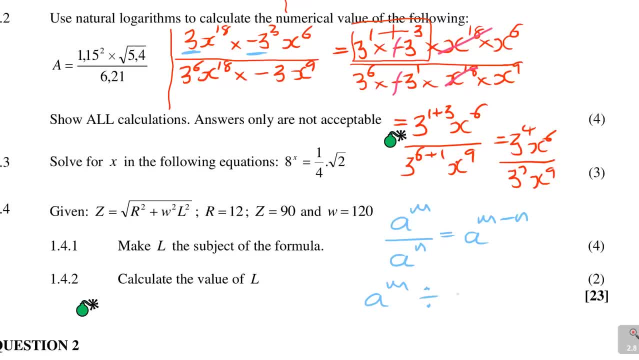 It is written usually like this: a to the power of m Divided by a to the power of m Is equal to that part. That is how they usually write it. So now, If I can use the same law here: 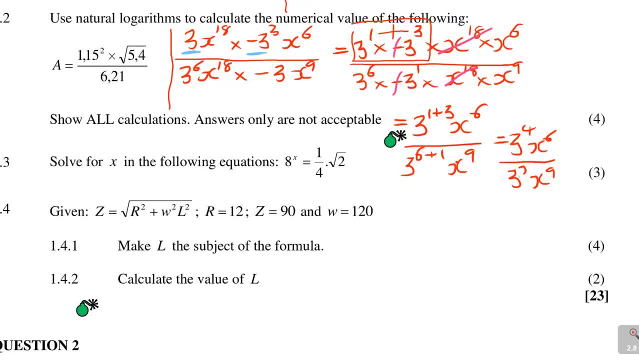 You can see, now I have got 3 to the power of 4.. x to the power of 7.. If you can look at that. So here I can apply that law and say This is the same as saying equal to. 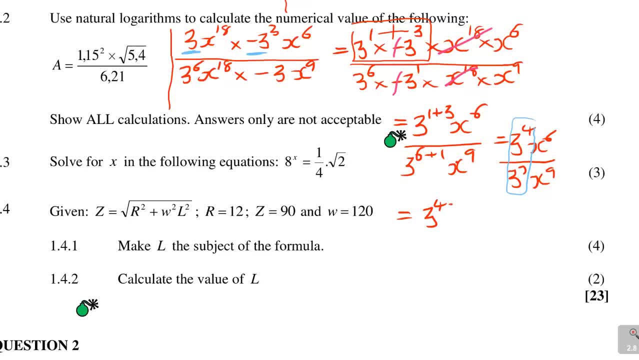 3 to the power of 4. Minus 7.. x to the power of 6. Minus 9.. Do you see that? So it will be 3 to the power of 4 minus 7. Is negative 3.. 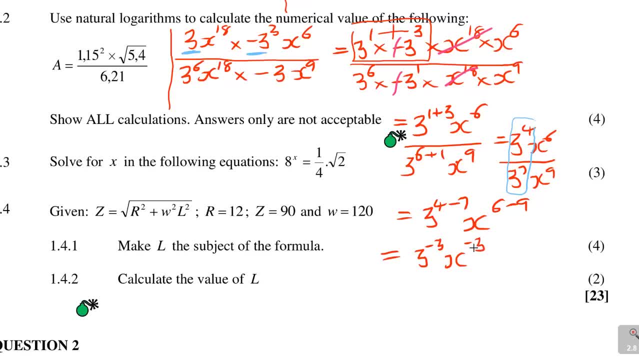 x to the power of 6 minus 9. Is negative 3.. Now, This is the answer, But it is up to you how you want to live it. There is also another law which says: If you are given a to the power of negative m. 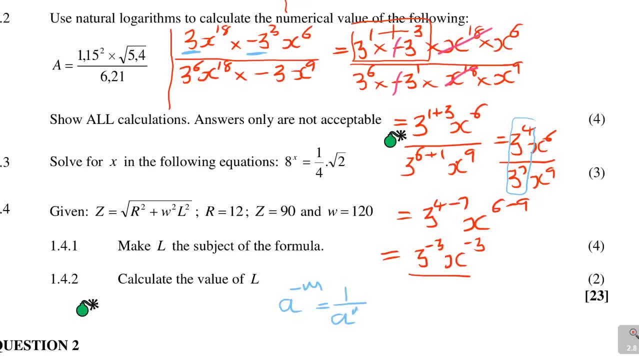 Is equal to. To get rid of that negative, We say 1 over a to the power of m. That is how you can get rid of that negative. So I can use the same here to say This is equal to 1 over. 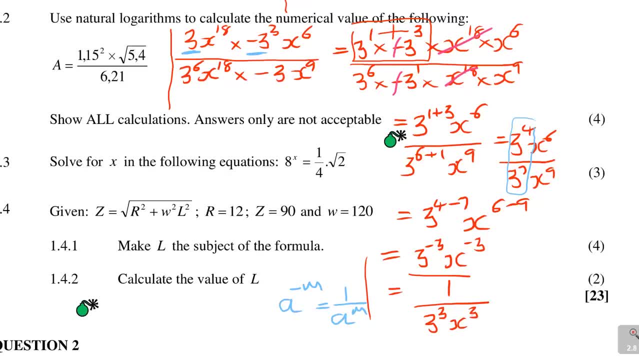 3 to the power of 3.. x to the power of 3.. So if I had worked it properly, This is supposed to be the answer, But I can test it Before I get the calculator. I usually prefer, as I say to my students, 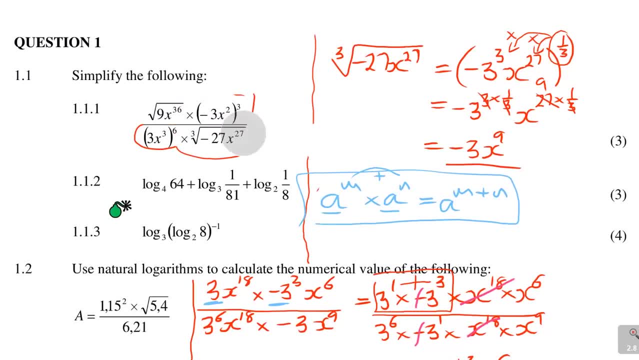 Always test your answers. It kind of gives you an assurance That you are in the right direction. I don't want to spend much time here, But it is always good to test your answers. I am not going to do it for now. 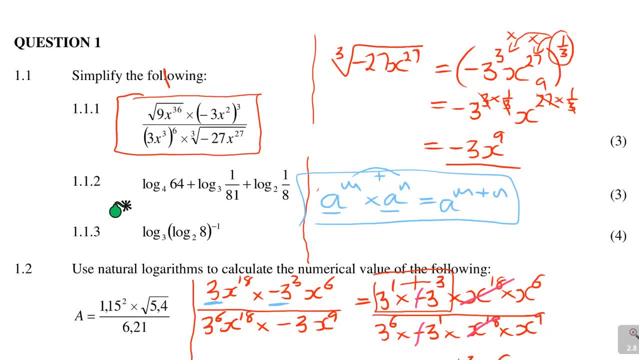 Because there is quite a lot of work to do. But what you do when you are testing here, You do this to say: Test your answer. Choose any value of x, For example. you can say So. wherever there is x, You put 4.. 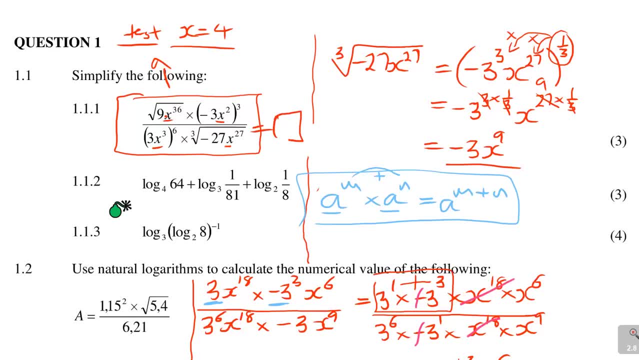 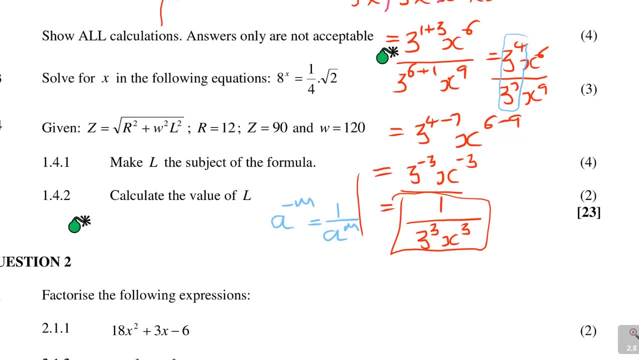 You put 4.. You are going to get an answer. You keep that answer. Again, you take the same value of x. Come and put it here Where? here You are going to have 4.. The answer that you got in the top. 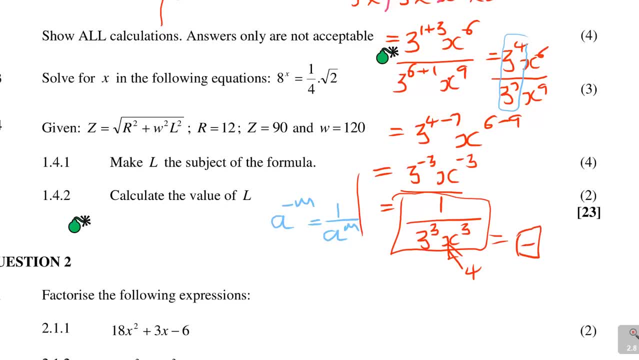 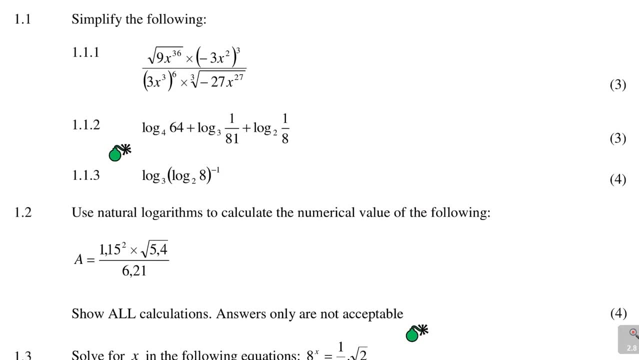 Must match the answer that you get at the bottom. If it is like that, It means your answers, I mean your solution is correct. So that is just that. I don't want to waste a lot of time, Let's look at 1.1.2.. 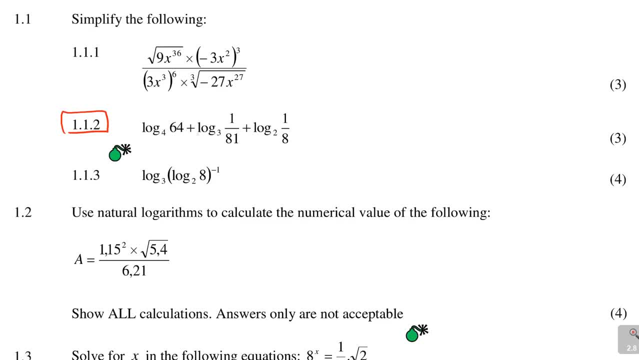 It says: log in base 4. Of 64.. Plus log in base 3 of 1 over 81.. Plus log in base 2 of 1 over 80.. It is 3 marks And they say: I need to simplify. 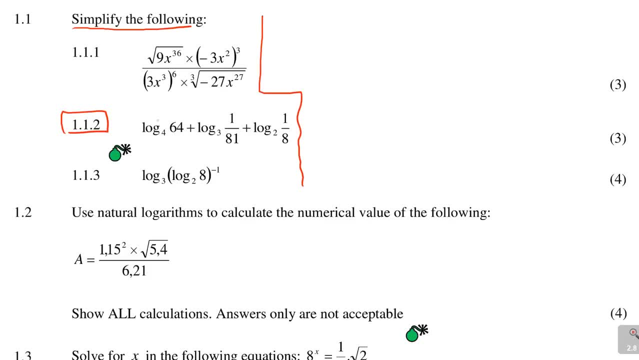 Again. let me just work this on here. Guys, Don't be in a hurry To try to solve this. Especially, it is 3 marks. Some students will prefer to do this. Let me show you what they will be tempted to do. 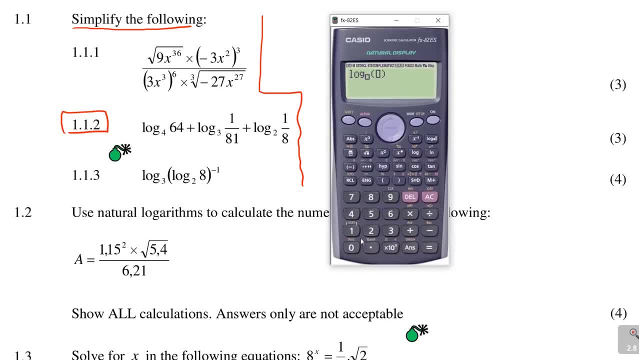 They will just take a calculator And say I can solve it. Then they will write log base 4. Of 64.. And then they will say plus Log base 3. Of fraction. There it is 1 over 81.. 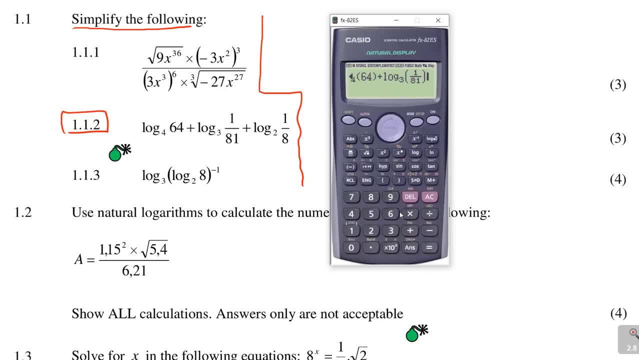 And then they continue To say: Plus, log in base 2. Of I think you can say it is 1 over 8. So this is what some of the students will just do, And then they get minus 4.. I know the answer there is negative 4.. 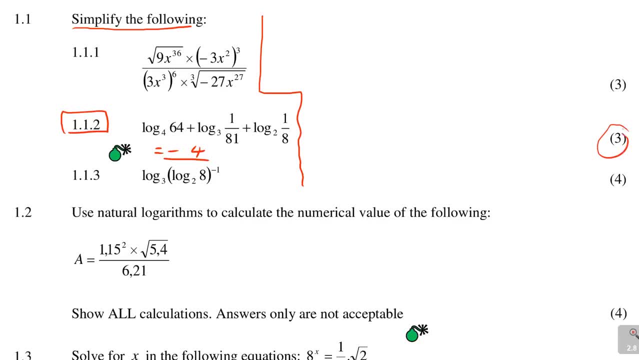 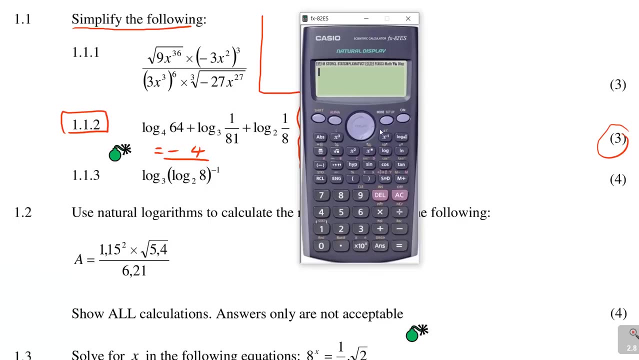 But, guys, You cannot get 3 marks out of that. What you need to do? You need to work smart, 3 marks Meaning you can still use your calculator In a way, In a clever way. You know what I mean. 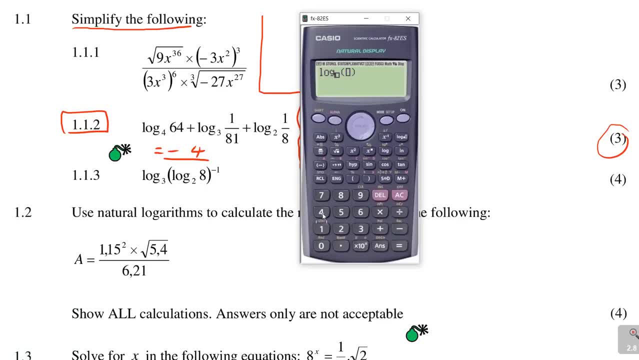 So when you use the calculator in a clever way, I am saying, let the calculator give you the answers And then work towards the answers. For example, It is 3. And then we will write 3 there, And then what is log base? 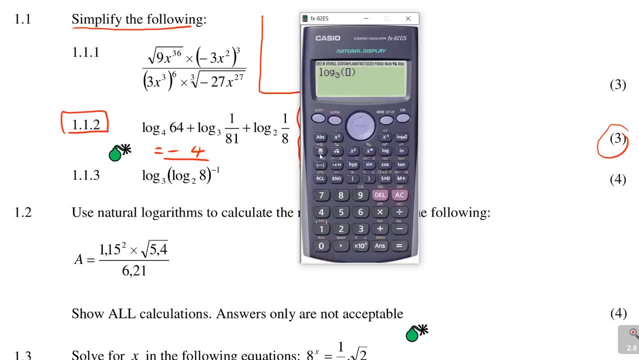 3. Of 1 over 81. You can see that It is minus 4.. So the first one is 3.. The other one is minus 4.. What is log? 2. Of 1 over 8.. 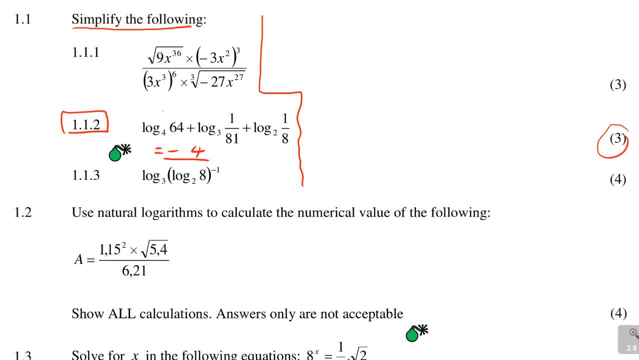 You see that it is minus 3.. So what we have here, We had 3., We had minus 4. And then we had 3.. So you just have to work and ask yourself: How did the calculator get these numbers? 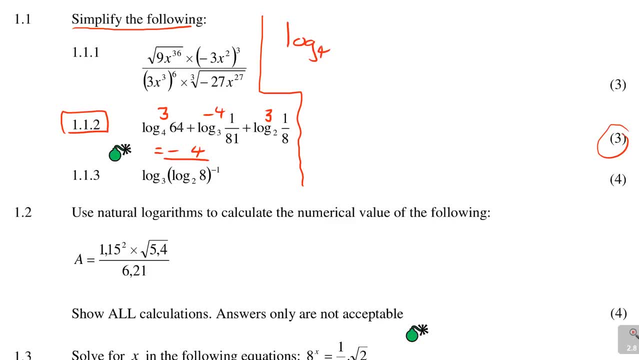 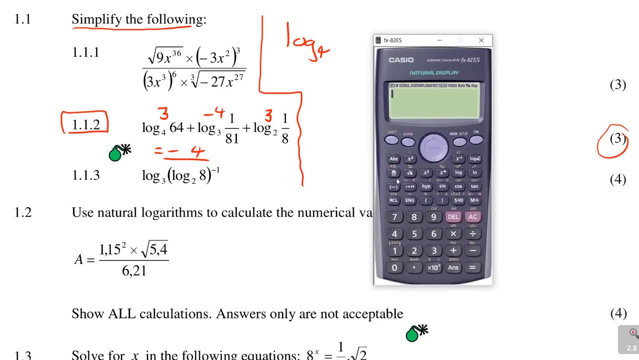 So what you do is, You know, log 4.. Now 64.. Using your calculator, It is always linked. These numbers are always linked. Ask yourself: How can I write 64 in terms of 4.. Try 4 to the power of 3.. 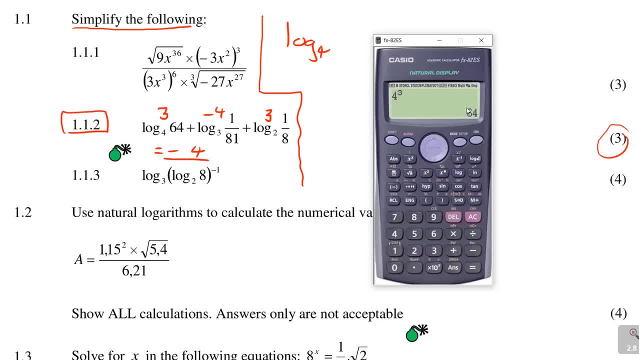 Already you know It is 16.. So to the power of 3 is 64. You see that, Again, 81 is always somehow linked To 3.. So how do you write it? Try, for example, 3 to the power of 3.. 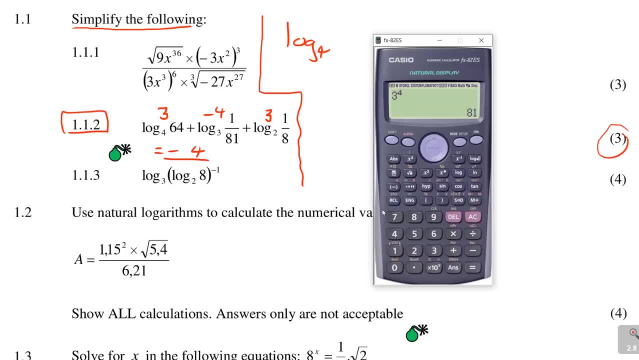 See, that is 27.. 3 to the power of 4.. You don't need to know the numbers exactly. So, to the power of 4, it gives me 81.. What about 8.? See, the base is 2.. Which means I must express 8 in terms of 2.. 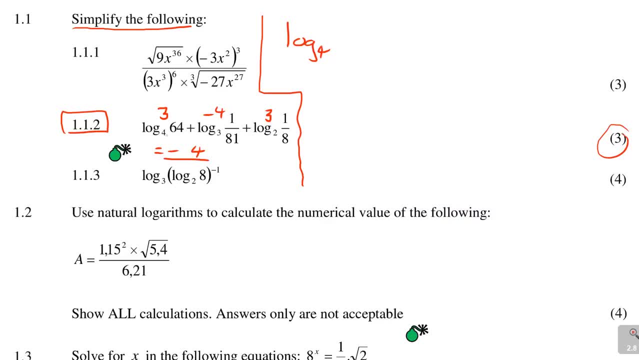 Which is 2 to the power of 3.. These numbers are always somehow linked, So I know 64 can be written in terms of 2.. But avoid 2. Because you are given a power of 4 there, So you need to in a way. 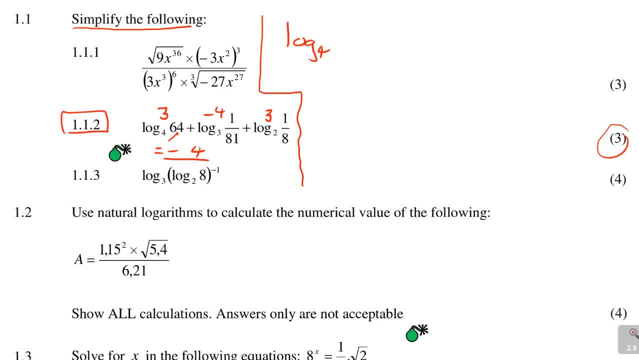 Work smart. What I can say is Always look where the examiner is taking you. So, which means, If they gave me a base 4.. I must express 64 in terms of 4.. So you saw that it was 4 to the power of 3.. 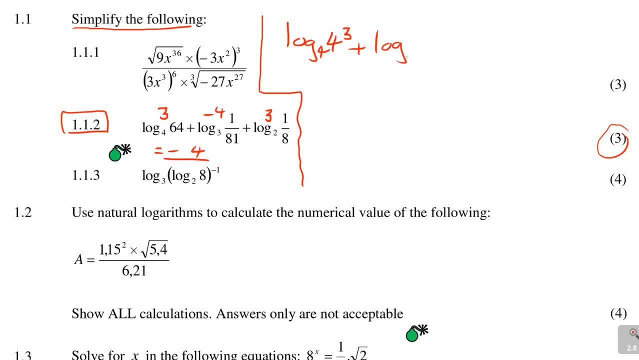 Again, plus Log base 3. 81.. 1 over 3 to the power of 4.. And then plus Log base 2. Of 1 over 8. You saw that it was 2 to the power of 3.. 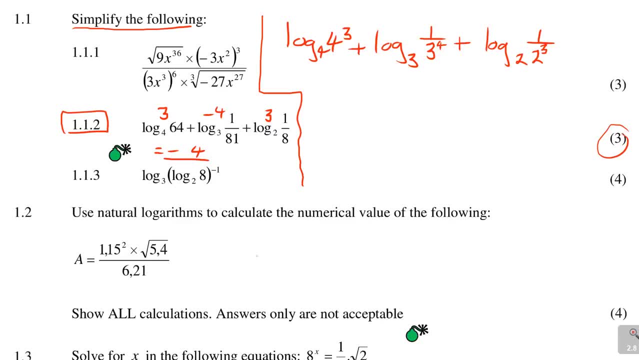 So we have done that. Now there is a law In logs And these things- Exponents, logarithms, They base on laws. So the law it says, If I can put the laws that I am going to use here, If I am given, 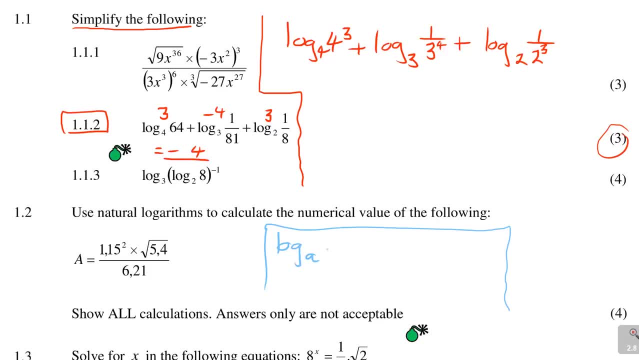 Log and base a. And then I have got M to the power of n. See that Now this particular n Will go down To become the n Log base a Of m. Remember this law. And then the second one that is going to be used here is: 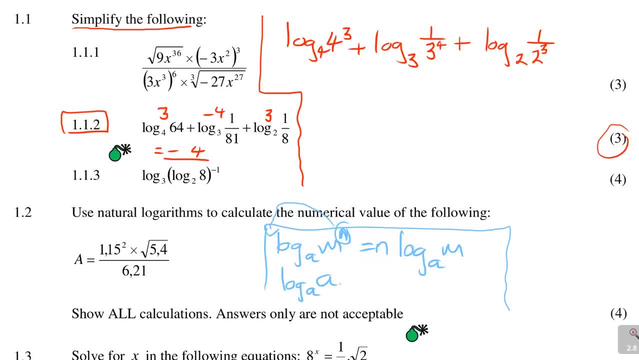 If you are given log base a Of the number a, If the base and the number are matching, You must know that that is equal to 1.. So those are the two laws that they want you to use there. So the first one here. 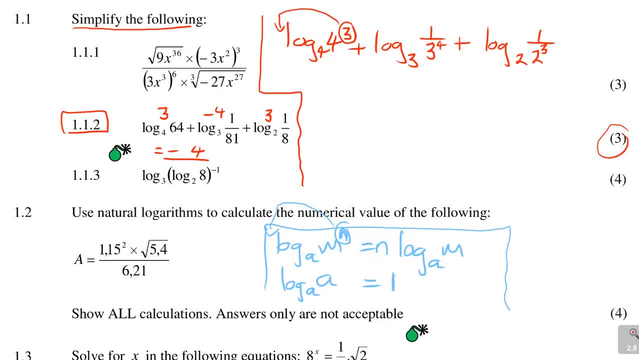 You can see the 3. Will go down there To become 3. Log base, 4. Of 4.. Plus again, I didn't finish, actually all the laws. There is another law Which says: If I am given 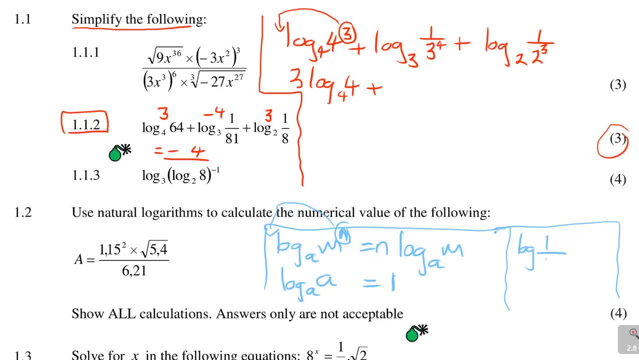 Log 1 over, For example, 2.. I mean, Let me use A to the power of m. See, that Is equal to. I can write This with the laws of exponents. Remember It is same as log. 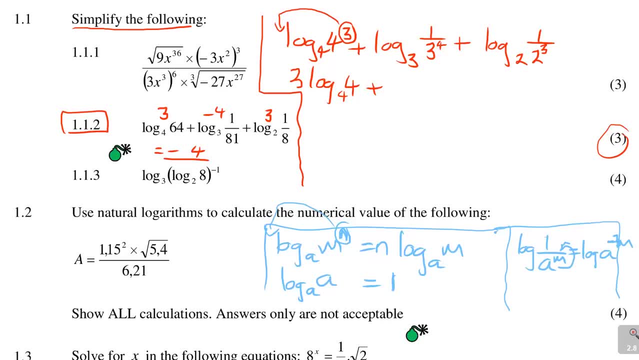 A to the power. Now, if this goes to the top, Is actually the laws of exponents I used? this one Is minus m 2 to the power, 4 to the top. It will become Log base 3.. Because of the division sign. 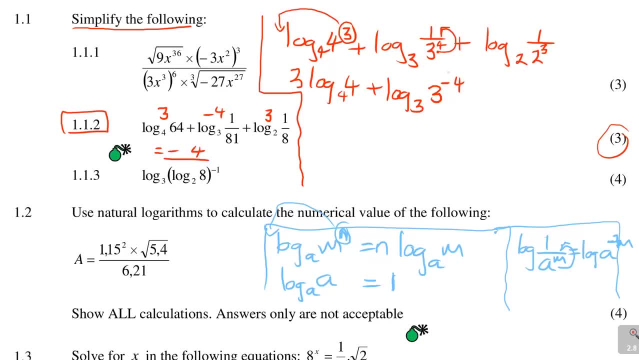 It will be 3 to the power of negative 4.. Just remember that If I want to get rid of this division line, I put a negative there, Ok guys, And then plus, Log in base 2.. I do the same thing there. 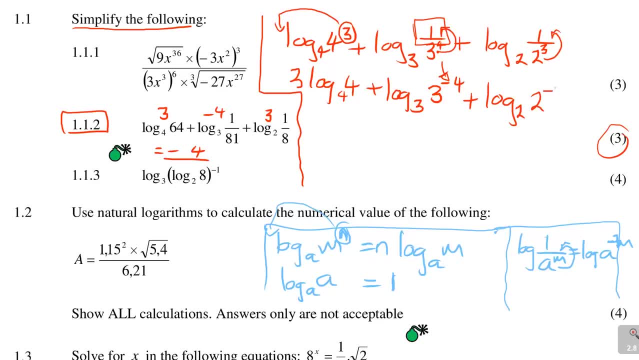 2 to the power of 3.. I want it to be on top, So it will be Now. I'm using then This particular law after that To say if the base and the number matching here- Look at this- 4, 4 so is 3.. 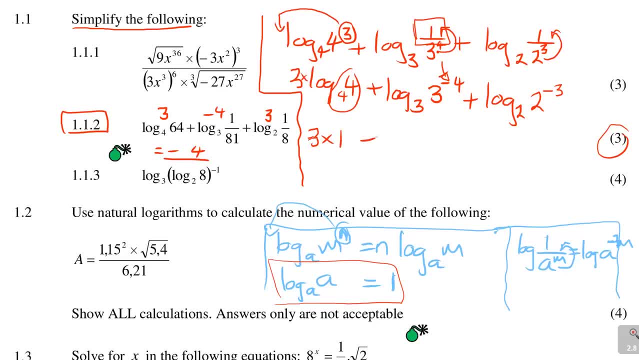 Now the 3 here is multiplying, So is 3 times 1, plus Again. Actually, before I do that, Still fine, Just leave it like that. Now this negative 4. Will drop down To become: I need to use a negative now. 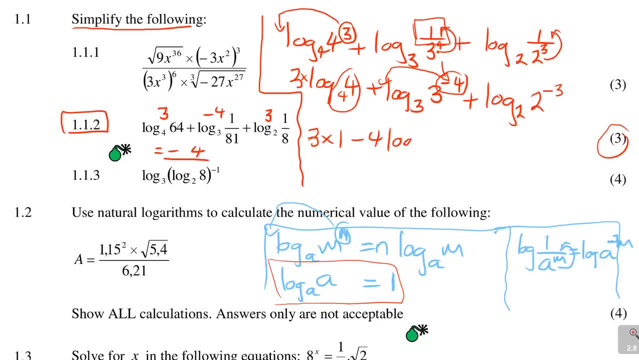 It's minus 4.. Log Base 3 of 3. Plus again This negative 3. Will drop down to become minus 3.. So I can actually Remove this particular Positive, because the negative Is more powerful, is minus 3.. 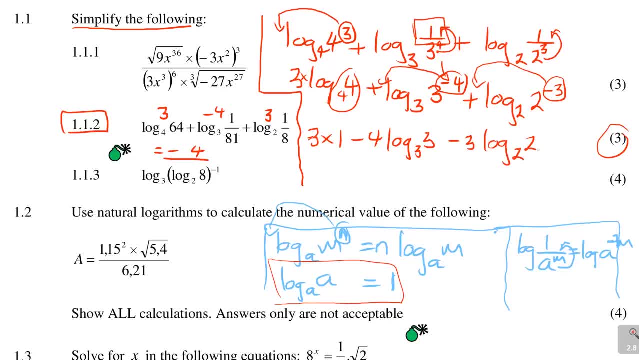 Log Base 2 of 2.. So now look at this again. The same law will apply here, Giving us 1.. So is 3 times 1.. Here Minus 4 times 1.. Minus 3 times 1.. 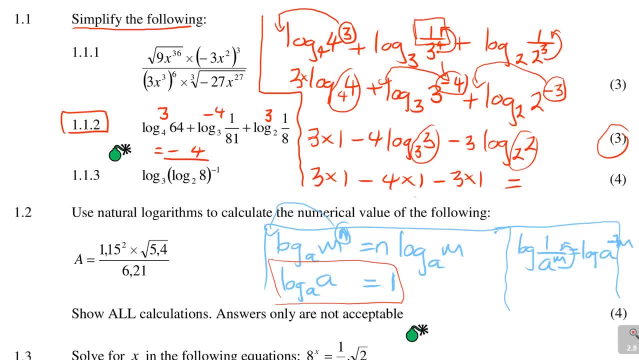 So when you simplify this 3 times 1. This will cancel that. You can see it's minus 4 times 1. Is negative 4.. This is what the answer Was given in that sense. So that is how some of these questions 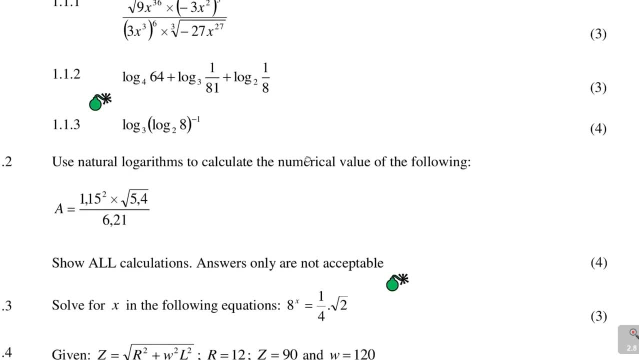 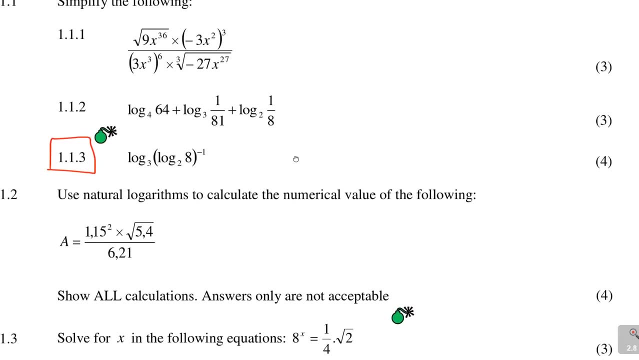 Are simplifying that. Okay, guys, I won't take long on that. Look at this one. I don't know why they gave it more marks. We need to be very sensitive in this question. It says Log base 3.. Log base 2 of 8.. 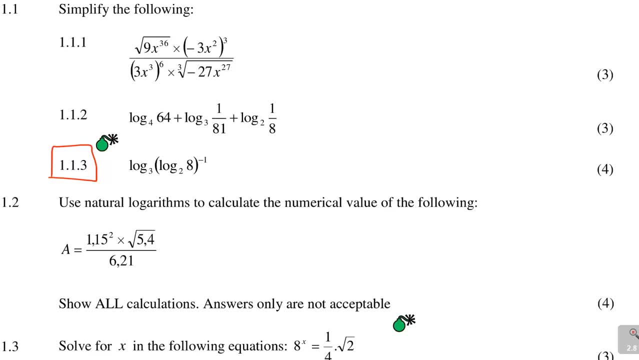 To the power of negative. 1. Don't get scared of such questions. You just need to ask yourself: What laws can I use? For example, Let me focus on what is inside the bracket. Of course you need to focus on the exponent. 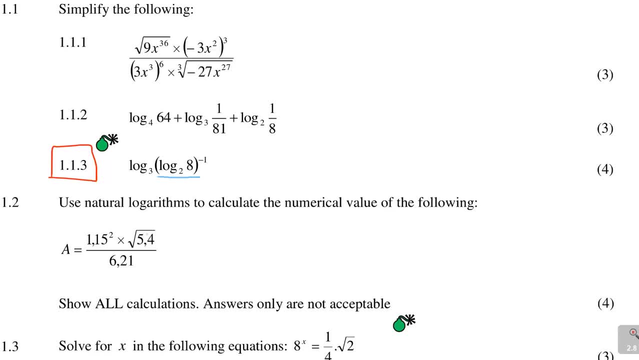 But I see two ways of doing this. one, Let's focus what is inside the bracket, Because there is always something That is common. Look at this Log. Oh, before we do that, Let's find the answer. It's always good with your calculator. 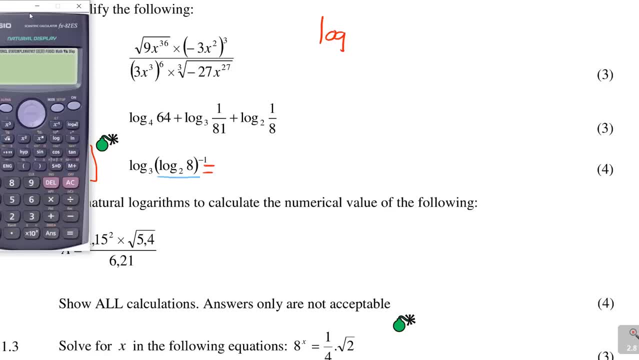 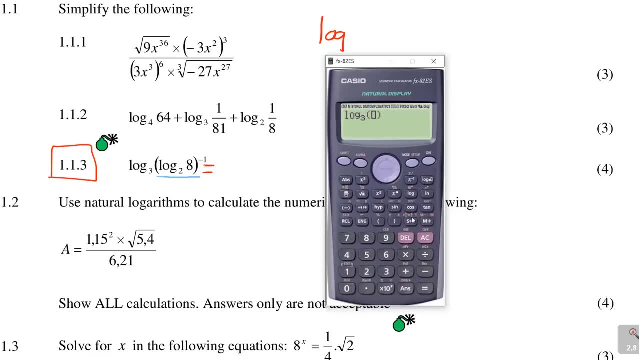 Work towards the answer. But remember there is not even a single mark you are going to get When you just use your calculator. Let's do it So it's log base 3.. There is the bracket. Again, I put a log base 2.. 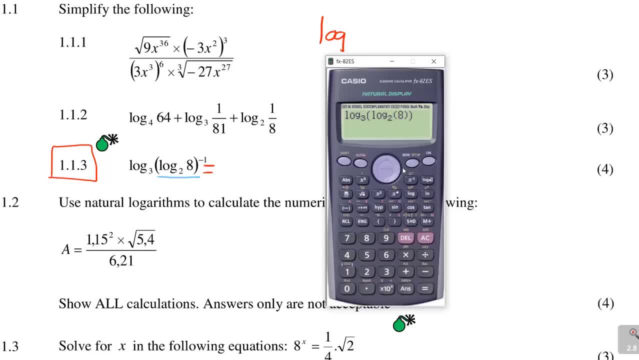 8.. Alright, So I must be very, very, very sensitive. So I put that, So that is that. And then, because if you punch it wrong, These things end up giving you wrong answers Like that to the power of negative 1.. 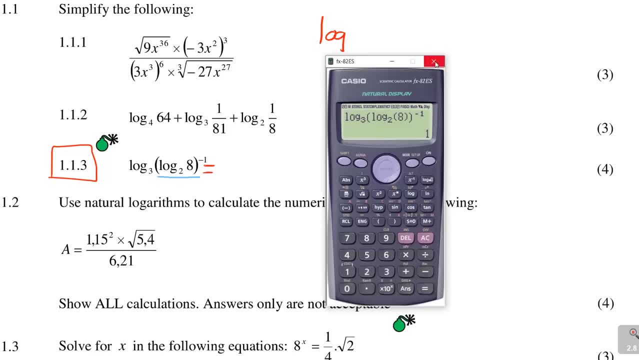 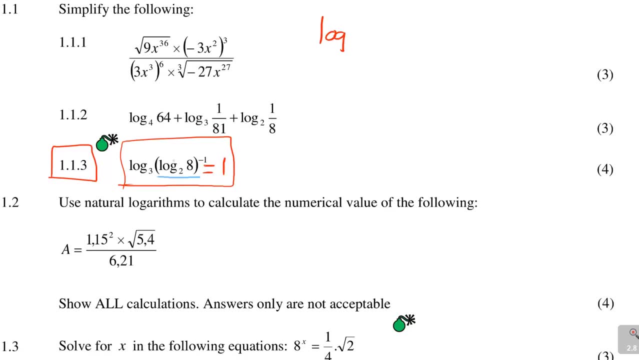 I'm getting a 1.. I hope I did punch this right, So let's try to get a 1 in this. So this is that: How did the calculator get a 1? So you know that you are waiting towards 1.. 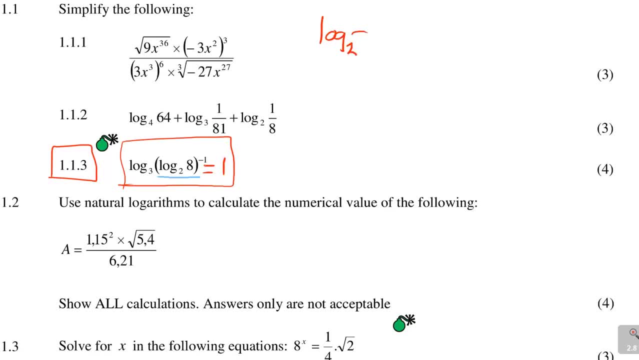 So let's try it. Log base 2 of 8.. I'm doing the bracket first, As we did. Using the law, We say this is same as log base 2.. 8 is 2 to the power of 3 guys. 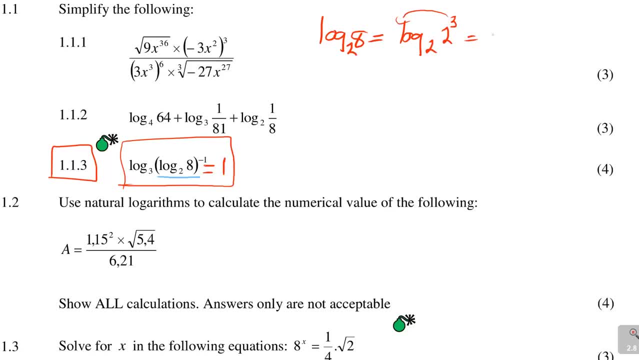 Which is equal to Take that 3 to the front, Which is 3.. Times log Base: 2 of 2.. Now, 2 of 2 is same as 1.. Remember, this is 3 times 1.. And the answer here becomes simple. 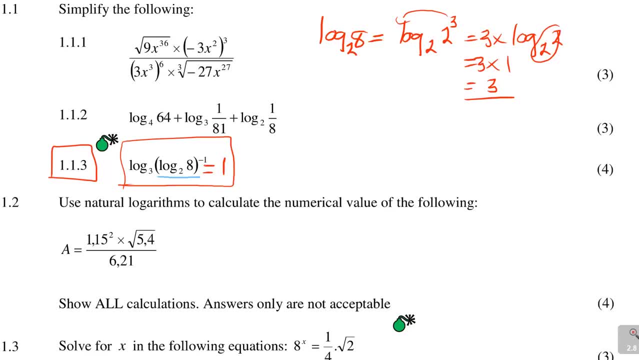 3.. So far, so good. We are done Now. which means this: You can now rewrite it as The same now to say: Log Base 3. Of 3. To the power negative 1.. Are you seeing that? 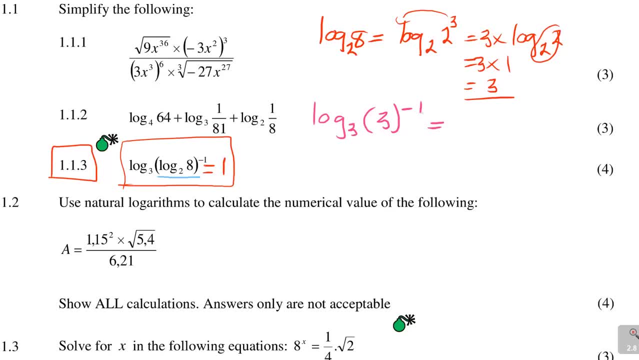 That is what simple means Now. it now simplifies So easily Because at the end of the day I can take this negative 1. Drop it at the bottom So that I've got minus 1. Log in base 3 of 3.. 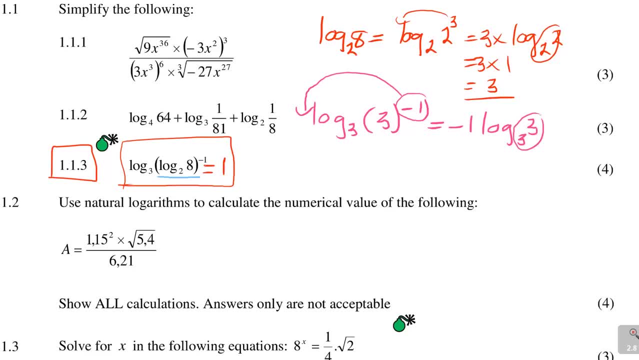 So that I've got minus 1.. Now log base 3 of 3.. You know what it is. It is 1.. So the answer is simple: minus 1.. I don't know why the calculator gave me a 1.. 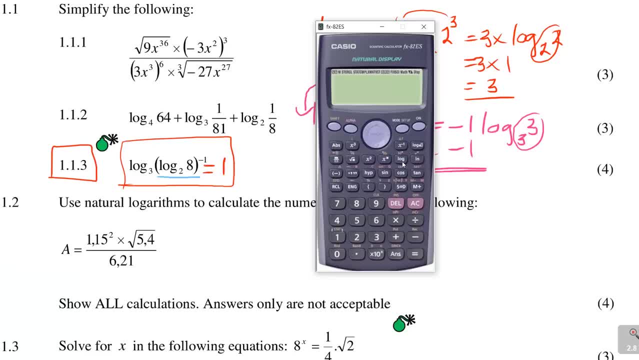 But let me try it again To see, if ever I didn't make an error. We say it: what Log base 3.. As I said, the challenge here is It will open its own brackets, So you need just to be careful. 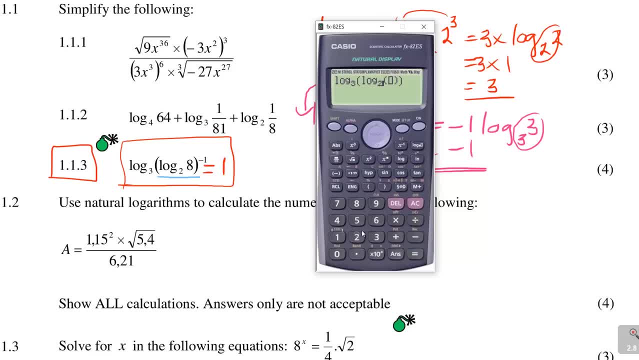 In the way it does. So I've got log And then I've got 8.. I think the power Is supposed to be there To the power negative 1.. You see, I put it on the outside, But if I put it on the inside, 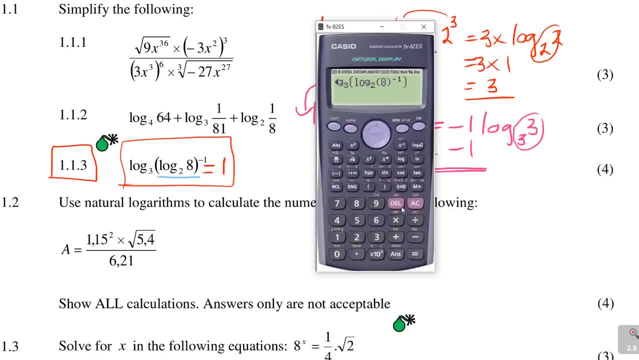 It is negative 1.. Do you see how this? you need to be sensitive, Because the calculator just opens its own bracket If I put it here And say to the power: negative 1.. I'm still getting a 1., But let me play. 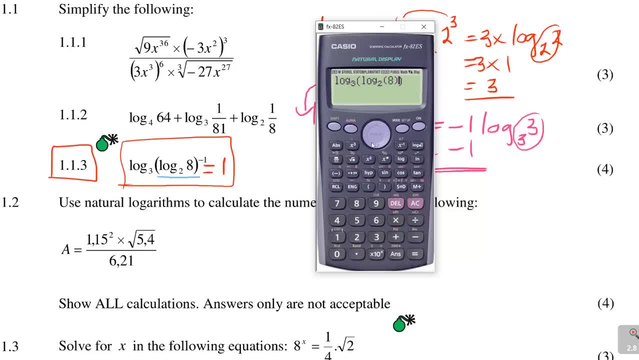 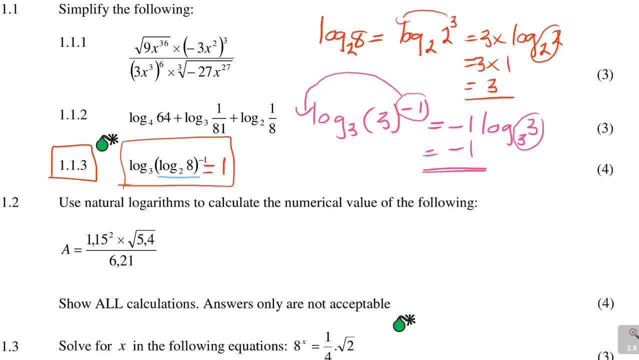 Back here And just put it inside here. To the power Negative 1.. See, you just have to be sensitive with the way the calculator does it. But even here Someone will be tempted to say But 3 to the power negative 1.. 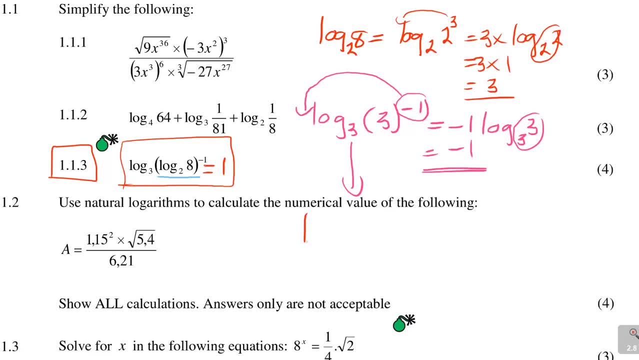 You could have taken it other way around. to say What if I wrote it like this: Log 3. Base 3.. 3 to the power negative 1. Is same as saying Log base 3.. 1 over 3.. 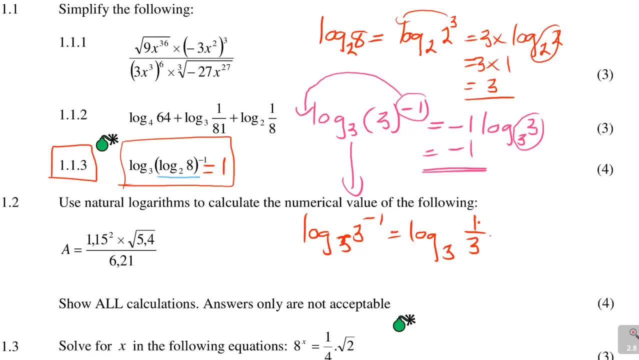 And remember that is 3 to the power negative 1.. It's still the same. You can apply the logs. If it's division, It means log base 3 of 1.. Division means minus Log base 3 of 3.. 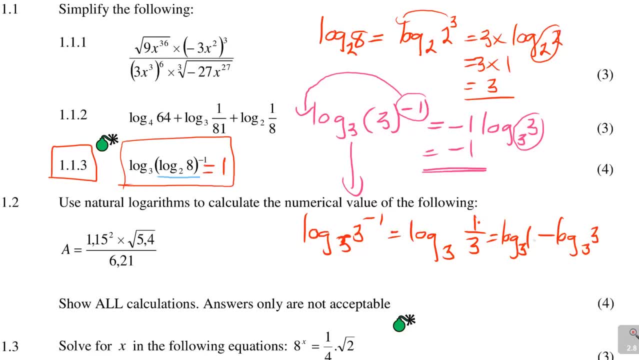 So you know that log 1. Is always 0. Log 1. Or any base. For example You can say log base a of 1. It's a log As long as log 1.. So even here This will become 0.. 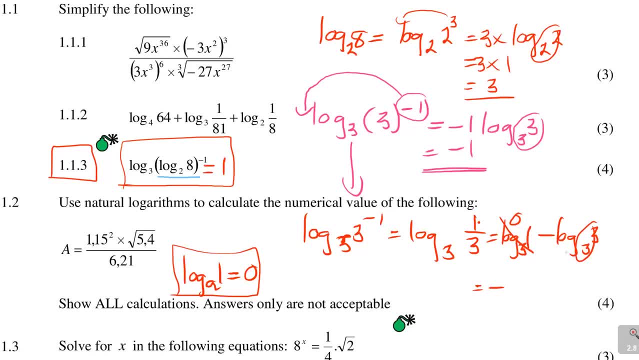 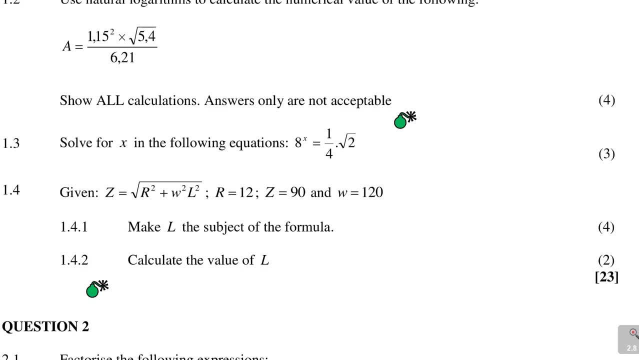 We have got minus Log base 3 of 3. See that, Which is negative 1.. So, whatever case You are still getting, the answer is negative 1.. Alright guys, So that was 4 marks, As I said. 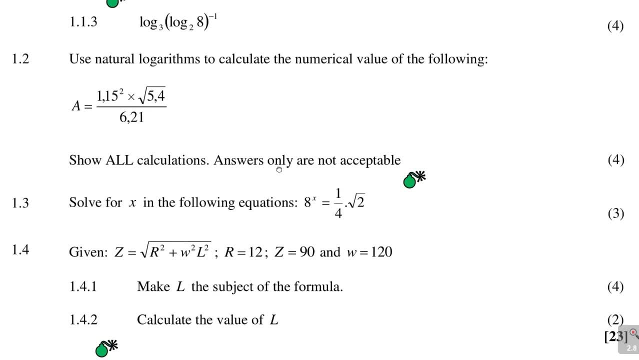 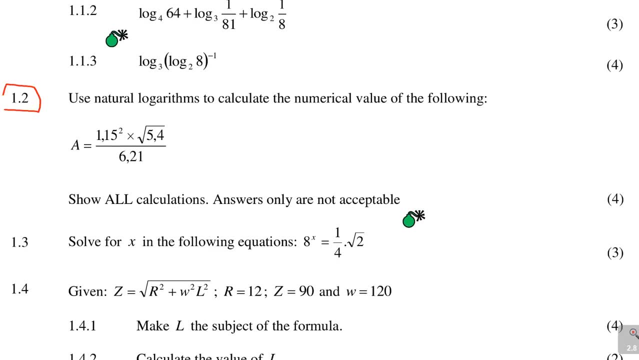 I don't know why they gave it, In a way, 4 marks, But I hope You have made it Okay. Number 1.2.. It's an important one, this one. guys, I will encourage you to master this. Just watch how I am going to solve this one. 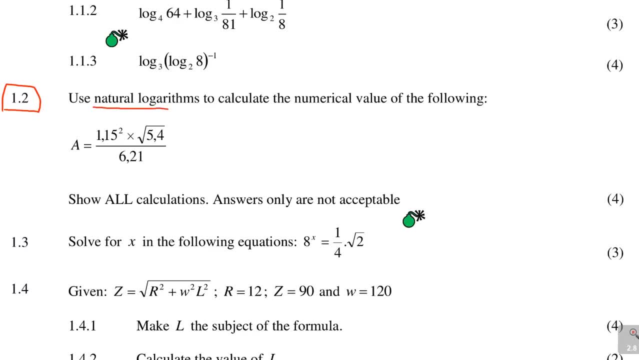 Because most students also they struggle When it comes to using natural logs. It says: use natural logarithms To calculate the numerical value Of the following: When they say natural logarithms, They mean lin. So you must use lin, Don't use logs. 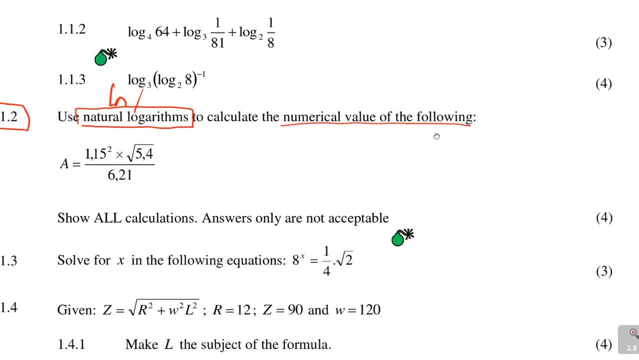 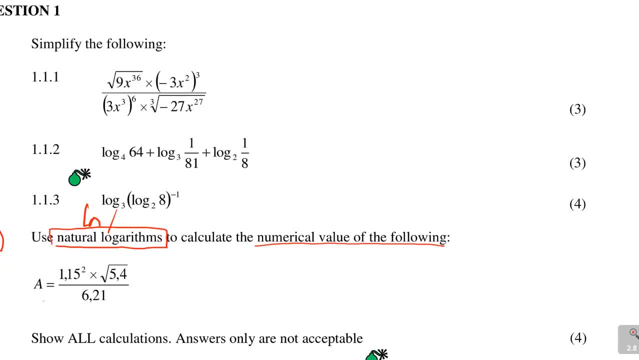 Natural logarithms Means you need to use lin. So what are they saying there? If you are saying use natural logarithms, I will just work from it here. So we are given this part. So the first thing that you do, Introduce the natural logarithms. 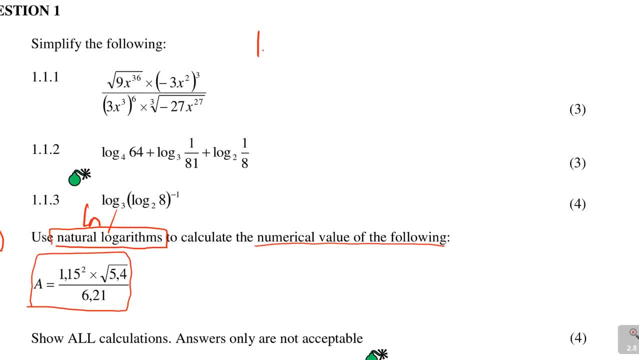 On both sides Where there is a. You just now say lin, a Is equal to. On the right hand side, also Put lin. You write everything as is 1 comma 1, 5.. Squared Times, Square, root of. 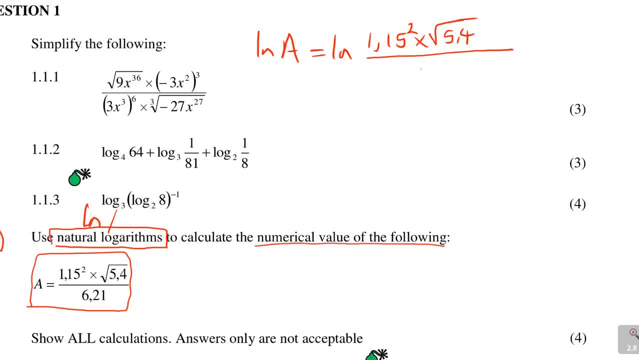 5 comma 4.. Over 6 comma 2: 1. That is what you do. Just introduce lin, That is the natural logarithms. Then, when you are at this stage, You need to now use the laws Of natural logarithms. 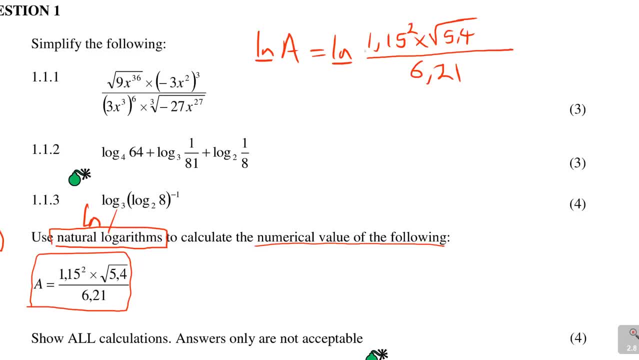 Don't be confused about this word: Natural logarithms. That is all The only difference between logs and lin. Let me come back to that to say: If you are saying, log The power, If it is on its own, If you don't put any power, 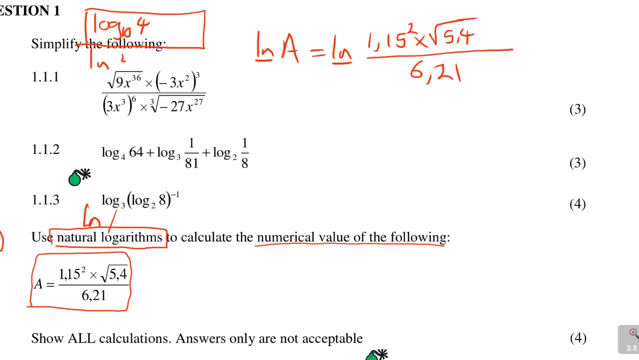 If I say log 4. The default is 10.. If I say lin 4. The default is e. So just the only difference there is: You are working with base 10., You are working with e. The calculator actually does have lin. 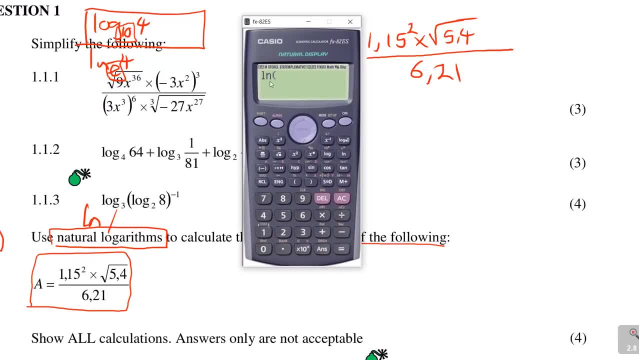 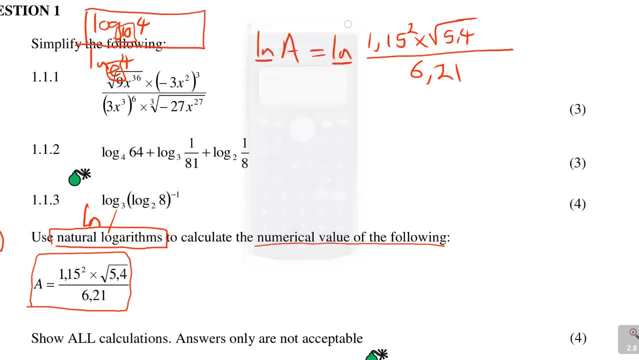 You see. So the moment I say lin, It means there is a hidden e, And in the calculator, the moment I say log, It means there is a hidden 10.. So you must always understand, But the laws are identical. So what you do is: 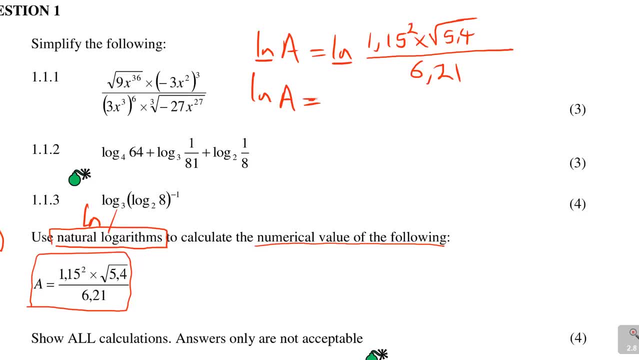 You continue with the left hand side as lin, a Continue with it. You also write here as the lin. Now you need to Kind of simplify some things. First thing is this: The square root. Remember the square means there is a power. 2. 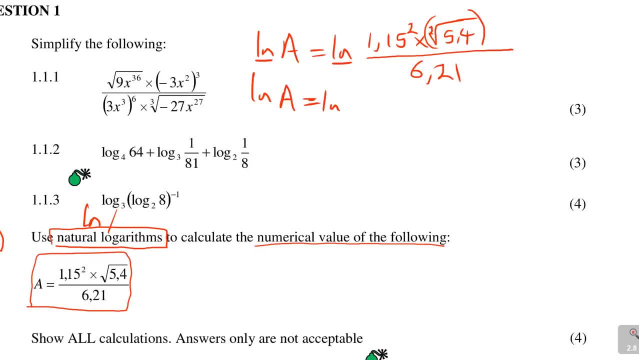 So you first simplify that It will be. Let me just use something much straighter, If I can have that. So what you will be having on top is 1 comma, 1, 5 squared Times. Now the square root. 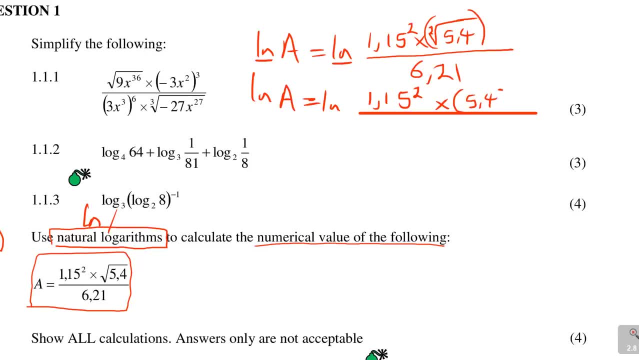 Remember you put a bracket, It is 5 comma 4.. And then it is power 1 over 2.. Remember that, Over 6 comma 2: 1.. Right, Again, I forgot something, And you know what I forgot? 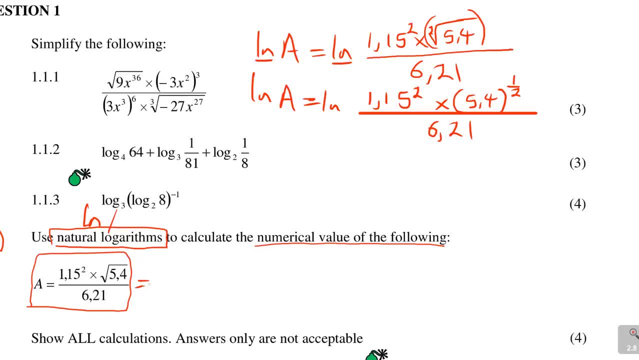 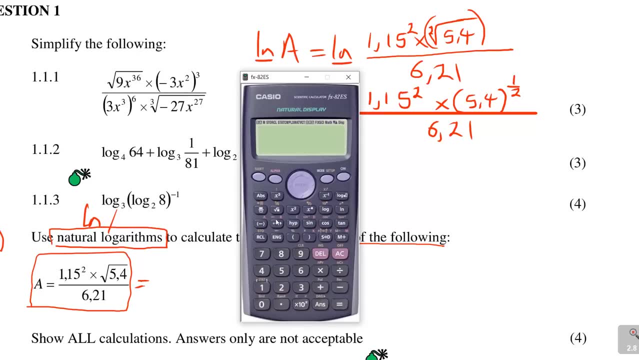 I forgot to first use my calculator, Because the calculator will always give me the answer. Let's find the final answer. this: Before we work towards it- I mean before we do any working- Always use your calculator. The calculator will just give us the answer. 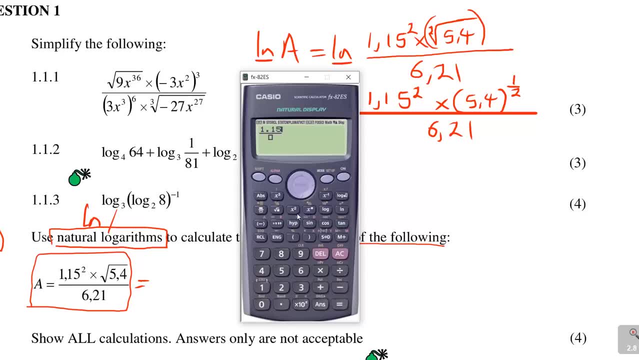 But they don't want you to use the calculator. Remember You won't get any marks. Square root of 5 comma 4.. And then I am saying Over 6 comma 2, 1.. So this is what I am having. 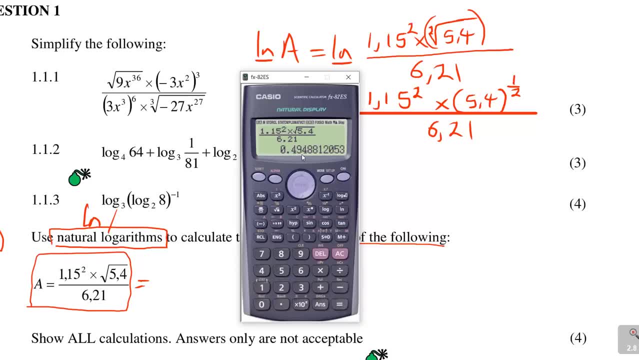 The calculator will give me an answer 0 comma 4, 9.. If I am leaving, I think the answers are supposed to be left to 3 decimal places. If they didn't explain, We will check the instructions again, But usually it is 2 or 3 decimal places. 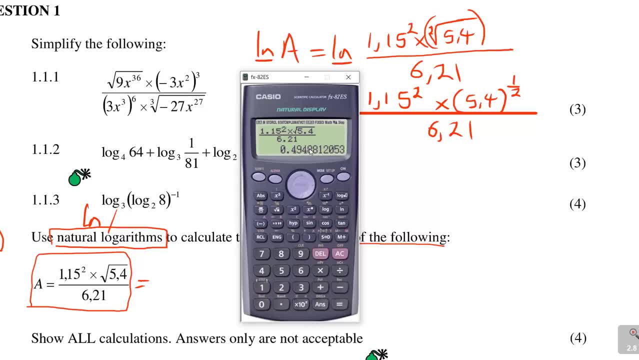 So if I leave this to 3 decimal places, It is 0 comma, 4, 9, 4, 8.. 8 will change to 4. 5.. But you can round off with the calculator. by the way You say shift Setup. 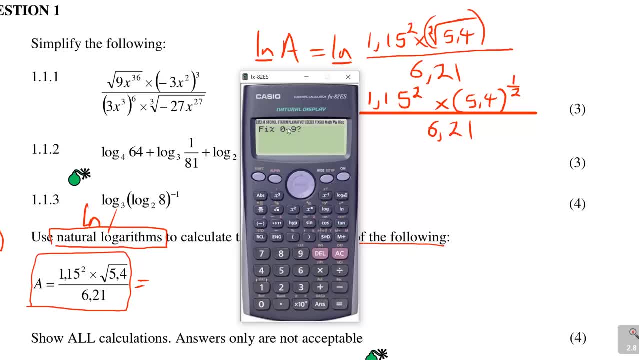 Then you come to number 6. there Fix, So you say 6.. Remember, I want to fix between 0 and 9. I want to fix it to 3 decimal places, So you say 3.. It is rounded off to 3 decimal places. 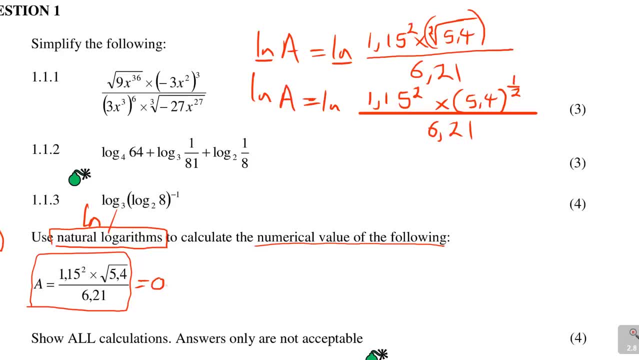 Which is 0 comma 4 9, 5.. So the answer is 0 comma 4 9, 5.. Guys, That's what I need to get on this, But in this case I am applying the logarithms. 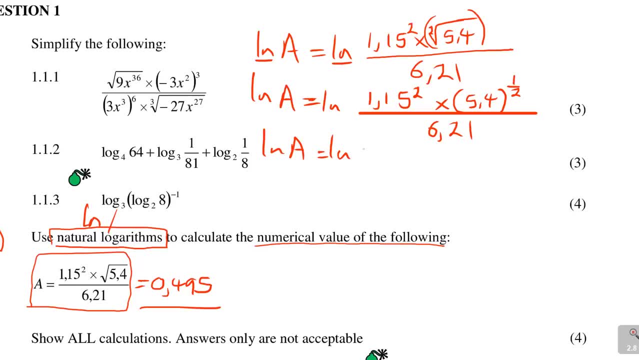 So I continue with my lin. a Is equal to lin. Now I am applying the laws. How do you apply the laws of logarithms When it is multiplying? You know that in the laws of logarithms you add, So what you have is: 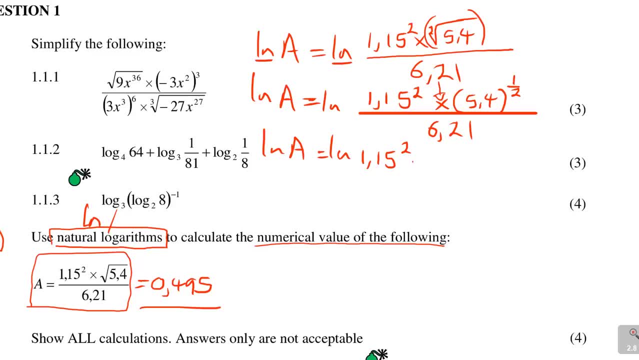 Lin 1 comma 1, 5. To the power of 2.. Plus, Because of the times, Lin 5 comma 4. To the power: 1 over 2.. So the division line means Minus: Lin 6 comma 2, 1.. 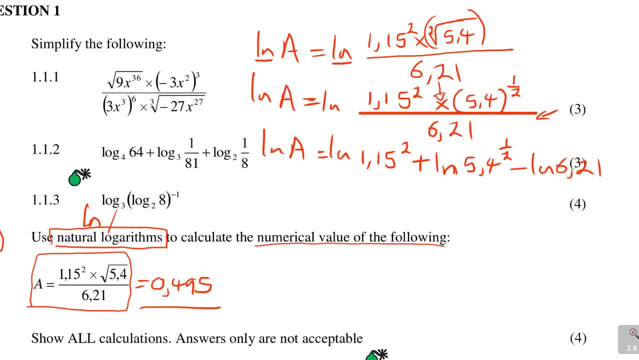 That's all that you need to know. When it is division, You subtract, When it is multiplication, You add. These are the laws of logarithms. Again, you continue. Lin a is equal to Remember the power. 2 drops down. 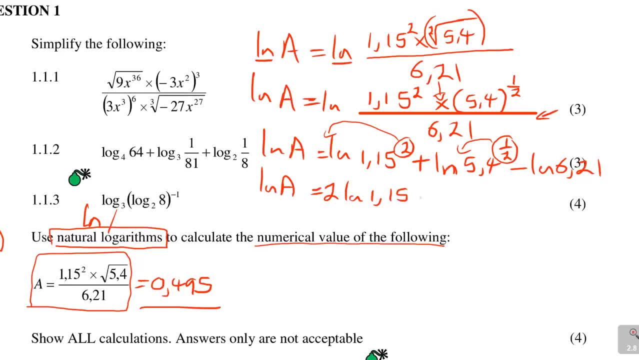 The half drops down. That's what you do: Plus 1 over 2.. In a way- remember it is multiplying Times: Lin 5 comma 4.. Minus Lin 6 comma 2: 1. That's what we are saying. 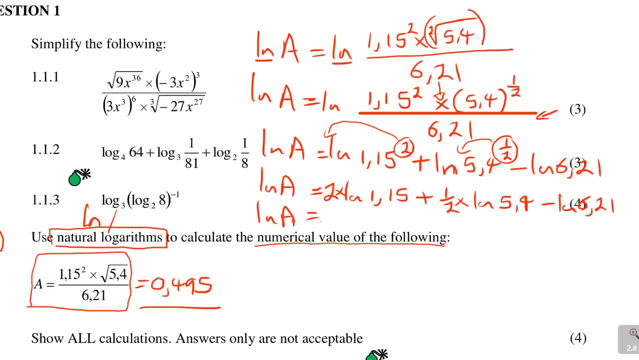 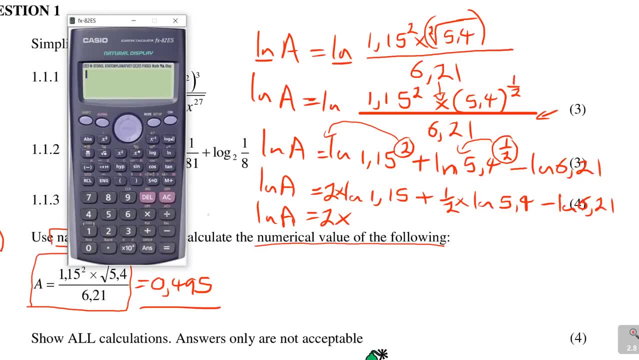 Now, by the way, you are Supposed to use a calculator at this stage, So you have got 2 times. Then you find what is Lin 1 comma 1, 5. If you are taking your answer to 3 decimal places, 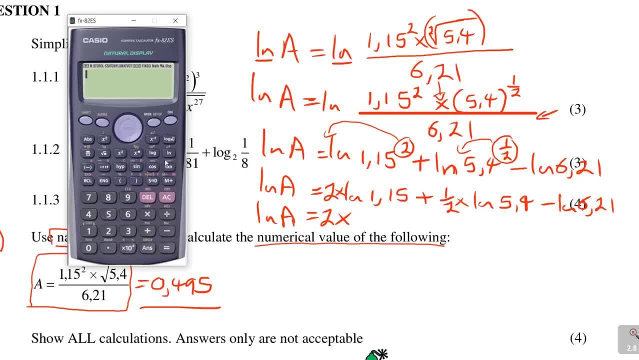 You can leave your answers to 4 decimal places So that when you round off It becomes 3 decimal places. So you come and say Lin 1 comma 1, 5. You need to definitely use a calculator here If I leave it to 4 decimal places. 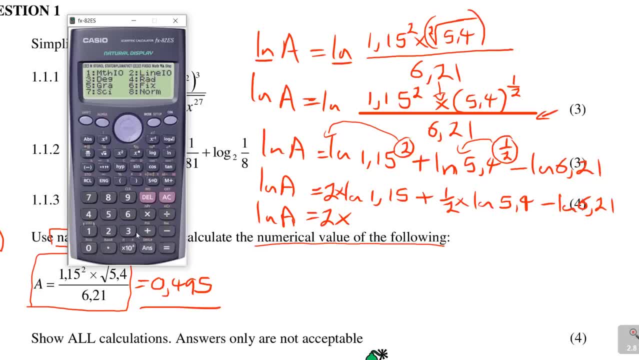 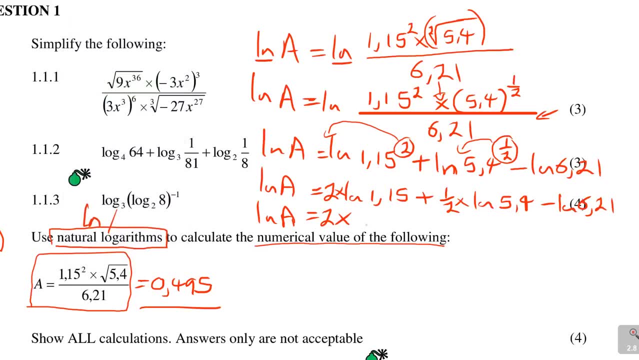 It is 0 comma 1, 3, 9, 8.. Remember shift 6 and 4 decimal place Is 0 comma 1, 3, 9, 8.. So 0 comma 1, 3, 9, 8.. 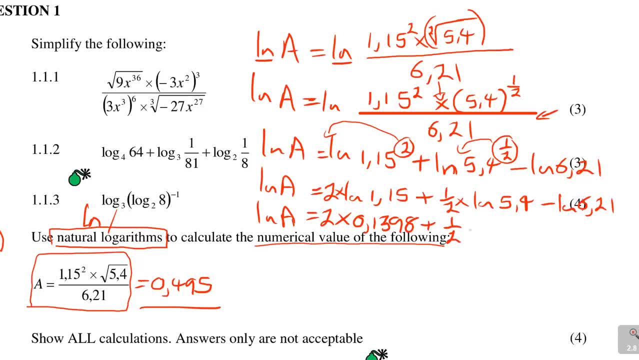 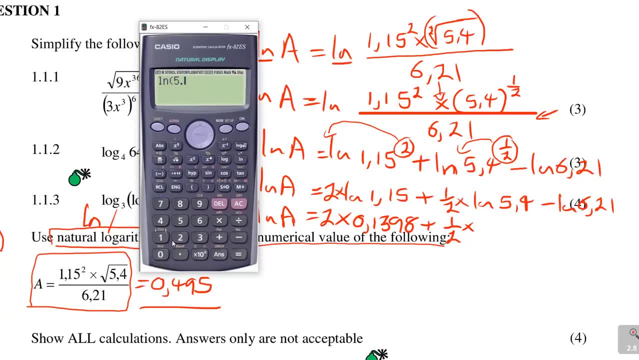 And then plus 1 over 2 times Again, I say Lin, 5 comma 4.. It will also give me The answer there. in 3 decimal place, Shift Number 6 to 4 decimal places Is 1 comma 6, 8, 6, 4.. 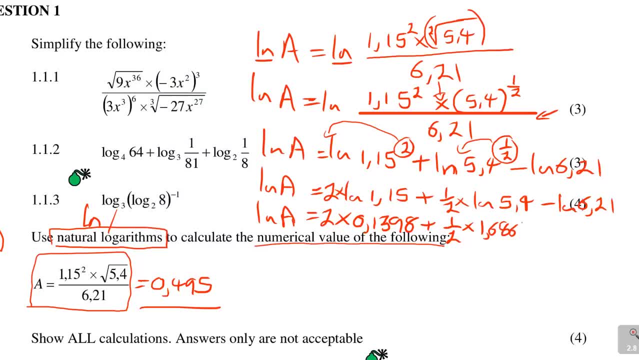 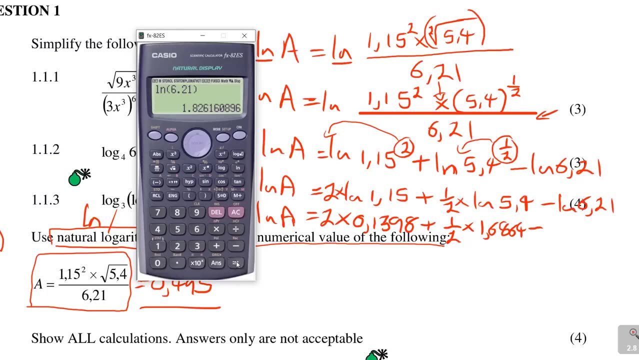 So 1 comma 6, 8, 6, 4.. Minus: The first one is Lin, 6 comma 2: 1. So Lin, 6 comma 2, 1. And then I am getting 1 comma. 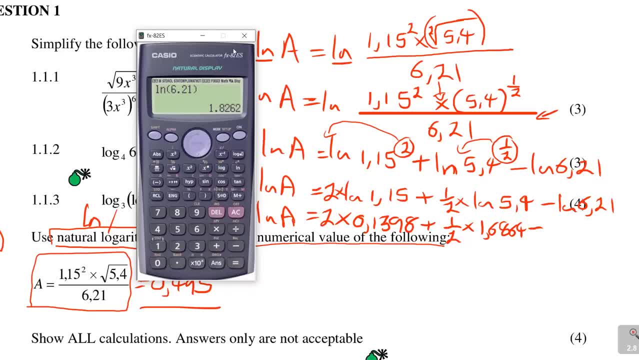 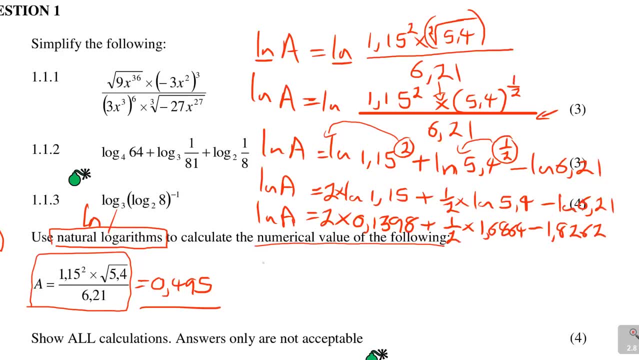 If I round it off again To 4 decimal place: 1 comma 8 2, 6, 2.. 1 comma 8 2, 6, 2.. At this stage, guys, I still continue. Lin A Is equal to: 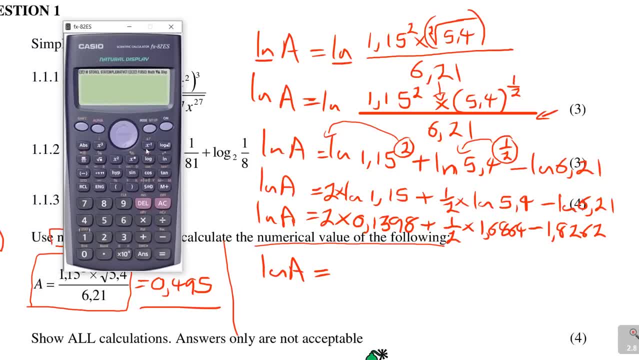 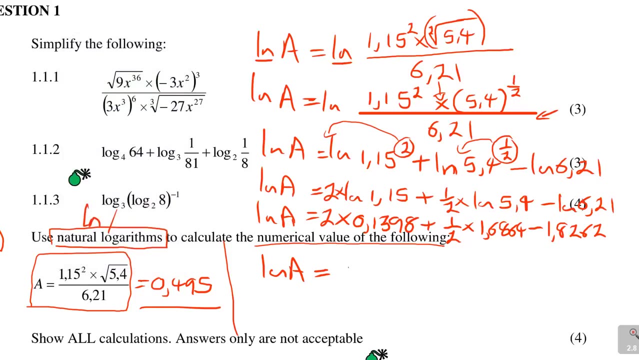 That by 2.. You know, I think you can see I am still relying on the calculator, But I am using the laws. So 2 times 0 comma 1, 3, 9, 8. It gives me 0 comma 2, 7.. 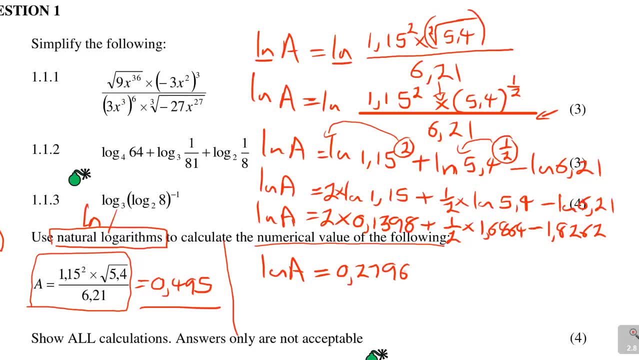 9, 6.. So it is 0 comma 2, 7., 9, 6.. But actually Let me not make this thing Too long out of nothing. Use your calculator Throughout now. So it is fine for me to come and say here: 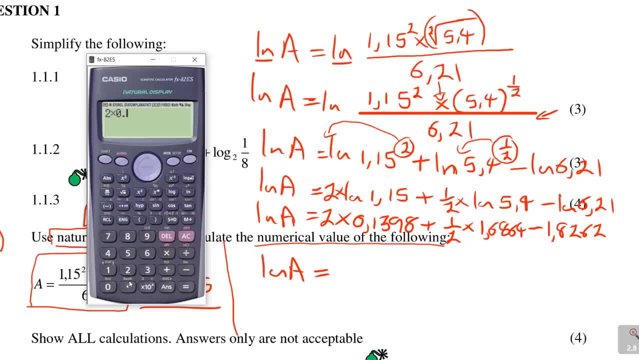 2 times 0 comma 1, 3, 9, 8. You can do that and say Plus half, Which is 1 over 2. Times 1 comma 6, 8, 6, 4. See what I am doing now. 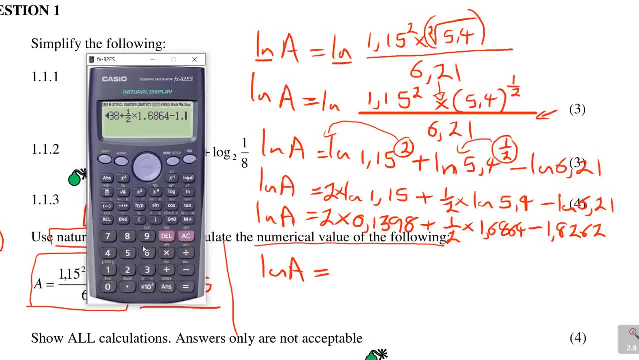 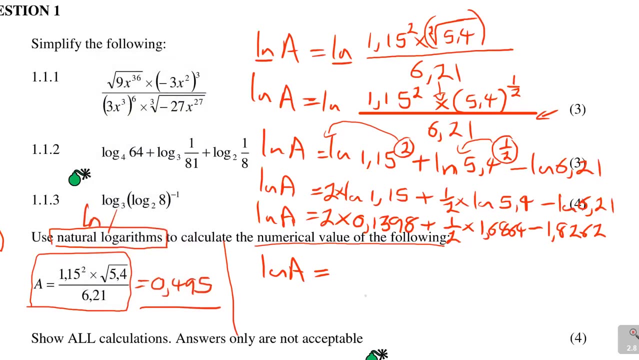 I am going straight: Minus 1 comma 8, 2.. 6, 2.. This is a lot Because you need to get, In this case, the final answer: Press SD. It is negative. 0 comma 7, 0, 34.. 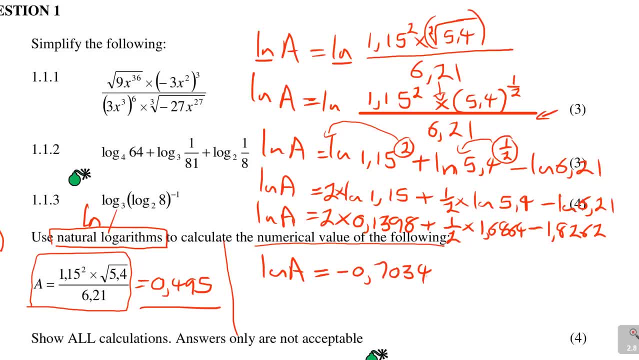 So it is negative: 0 comma 7 0 34.. At this stage You need Actually there is, If you Remember, I was already. It is now you to find The final answer. I say to you: Whenever you are given lin. 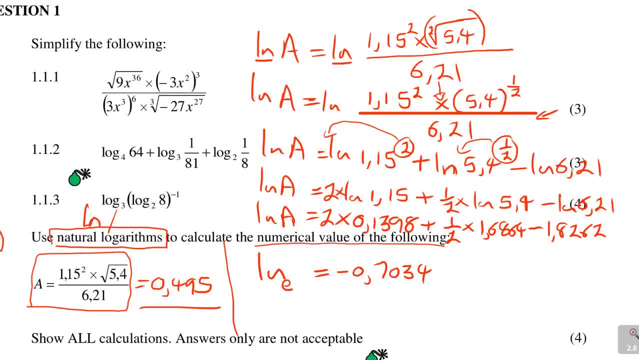 Here You must know the default base, Default base, is what It is, e. So lin in base e of a That you need to remember. So how do I then get my a? Because the question was: Use natural logarithms to calculate. 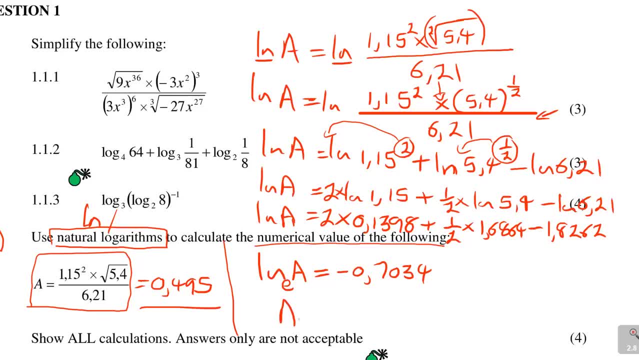 The numerical value of the volume. So they want the value of a Is equal to. You take that e to the power Negative 0 comma 7 0 34.. That is how you write the final answer: Equal to. 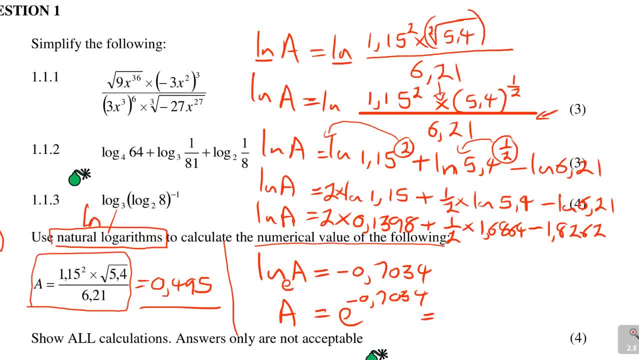 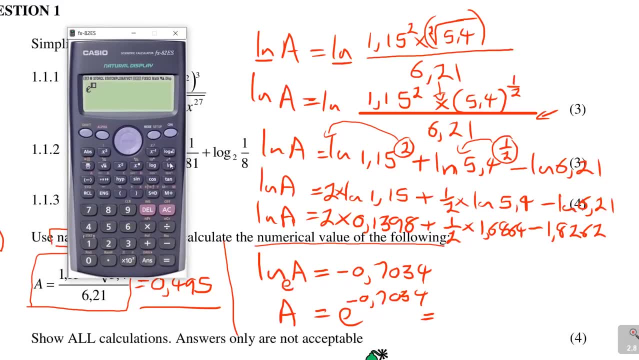 Again, the calculator is your, So it will give you In a way The final answer. So how do you find the e? It is shift e And then you have got negative, 0 comma 7, 0, 34.. 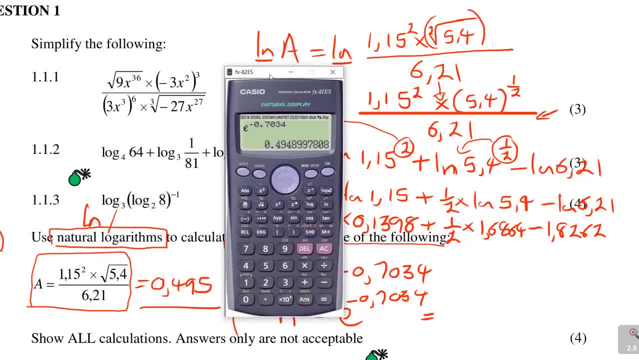 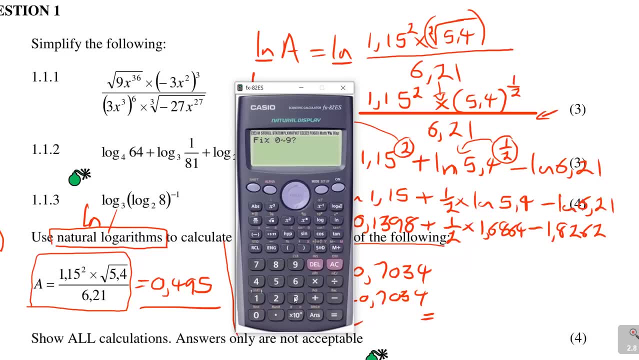 There, the answer is It is 0 comma. Let's compare it with what we have: It is 0 comma 494899.. Shift set up to 3 decimal places. There it is 0 comma 495.. What we just got. 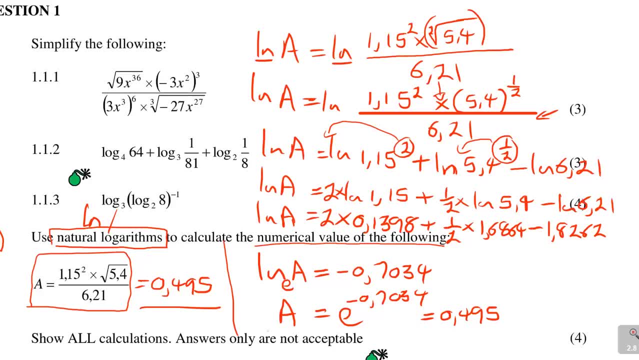 Which is equal to 0 comma 495.. So, as I am saying, guys Know where you are going. Don't just answer for the sake of answering. You get your answer. You are satisfied with the answer Which you have actually tested. 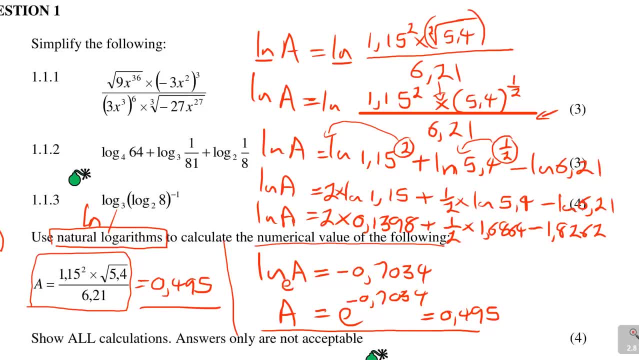 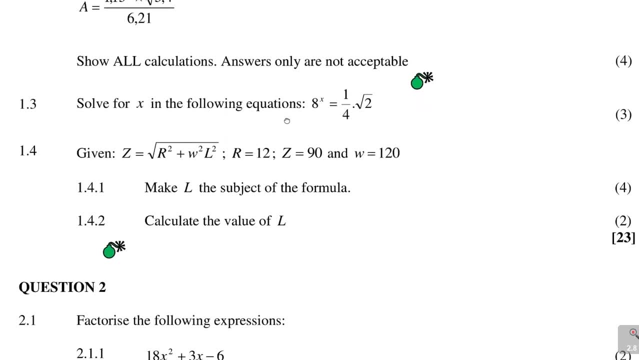 So you can see that Almost in all these I can actually use my calculator To first find the answer And then work towards that particular answer. Alright, so 1.3.. I am just about to finish now. Just I know it is late. 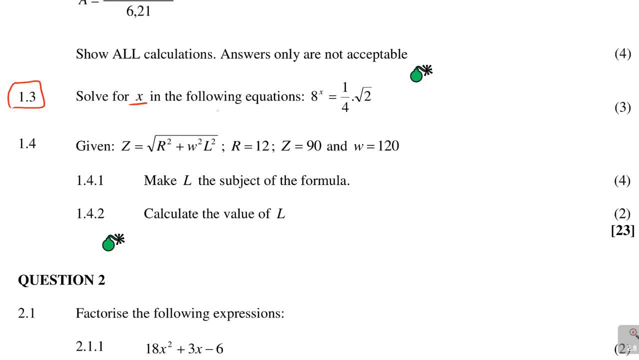 But just keep with me, I am just wrapping this up. So you solve for x in the following equations And I am given that Again, it is how many marks? This is 3 marks, So I don't think it was much of a problem there. 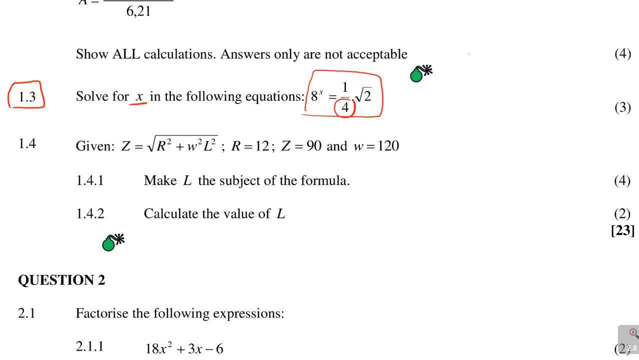 First things first. 1 over 4.. You needed to know that. 1 over 4. Is same as saying 1 over 2 squared. You see Which you take it to the top. It is 2 to the power of negative 2.. 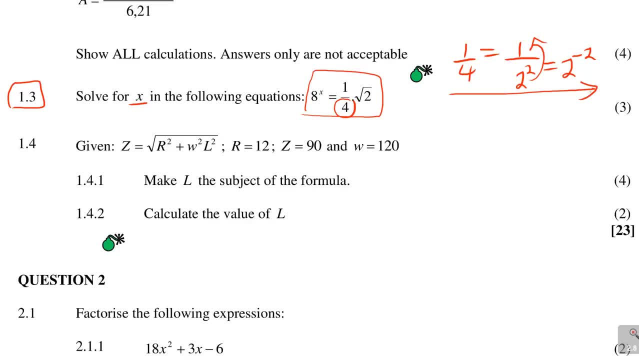 Such things you need to know, Such things you need to know. Secondly, Square root of 2.. I told you, square root means bracket. There is a hidden 2 there, So you have got 2 to the power, 1 over 2.. 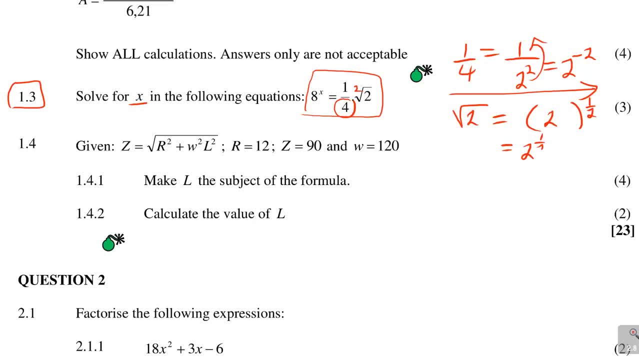 You can just simply write it like this: 2 to the power, 1 over 2.. You understand. So these things, you need to already have them. So if I write it again, 8.. 8 is same as If I say to you: 8.. 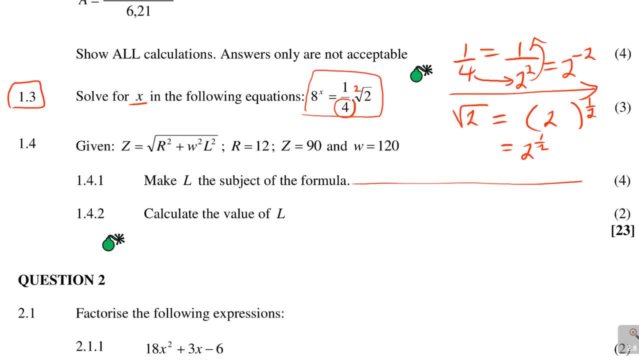 You need to see already 4.. I have transformed it in terms of 2.. Square root of 2 is now in terms of 2. Which means I must also change 8. To the power of x Into A base of 2.. 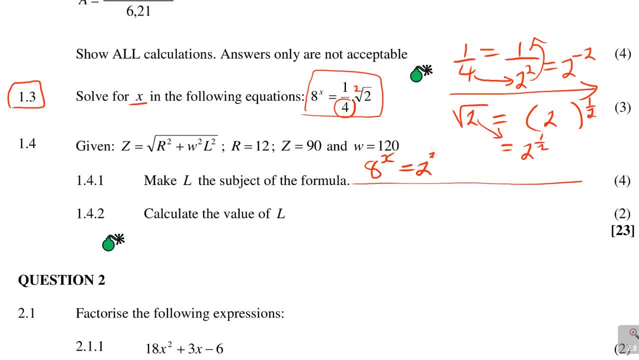 So 8 is same as 2 to the power of 3.. So that is the 8. But you put a bracket, You put the x there. So when you write this, You are going to say 2 to the power of 3.. 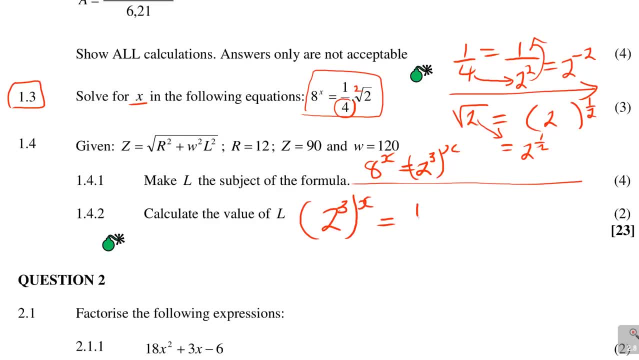 X Is equal to 1 over 2 to the power of 2.. Times 2 to the power of 1 over 2.. That is the first important step. Then, you know, 2 to the power of 3x. 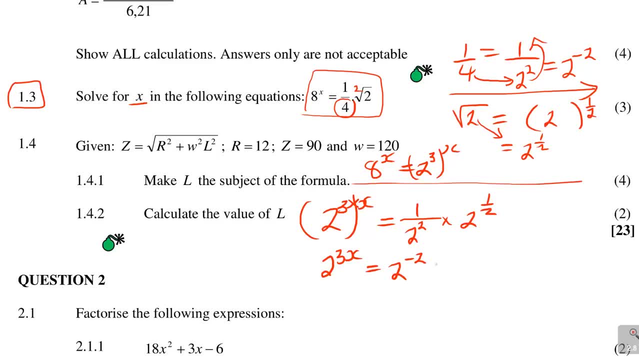 Is equal to 2 to the power of negative 2.. Times 2 to the power of 1 over 2.. See that You are simple using now. It is an equation, But the laws of exponents are very, very valid in that case. 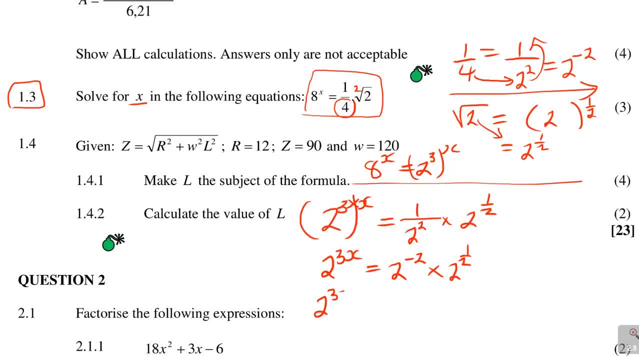 Now look at this other part. So 2 to the power of 3x Remains as is. But you need to focus here. The base is the same, So you need to add the exponents If you are given a to the power of m. 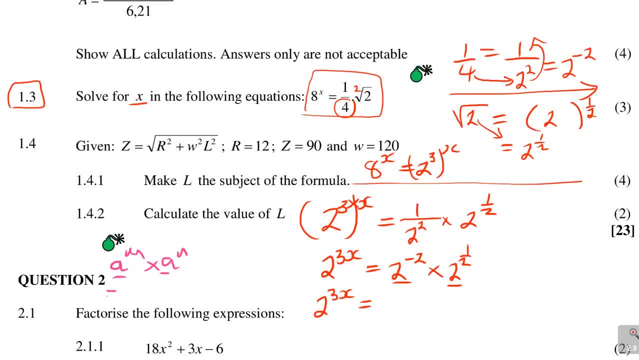 Times a to the power of n Bases are the same. This is equal to a to the power of m plus n. So even here The base is 2 and 2.. So it is 2 to the power of minus 2 plus 1 over 2.. 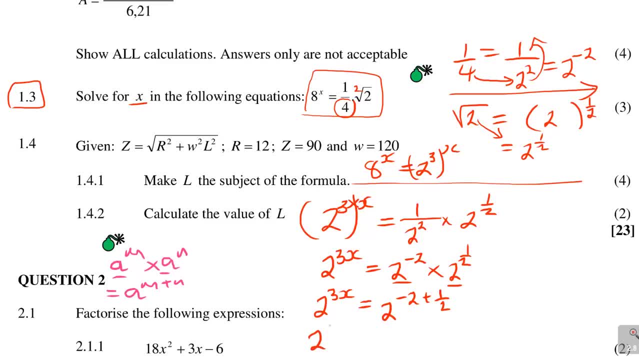 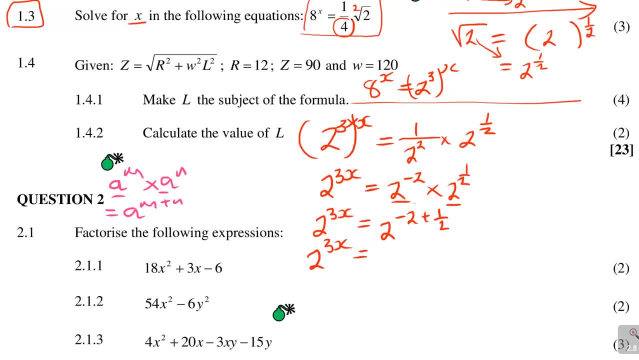 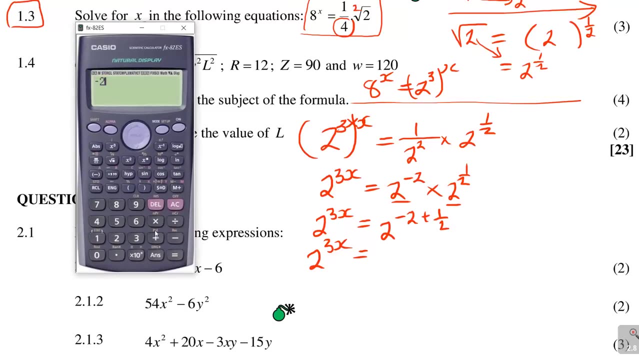 I think that So you have got 2 to the power of 3x Is equal to: Just to continue working on this, It will give us minus 2 plus half, I think, Negative one and a half. But then we just use a calculator. 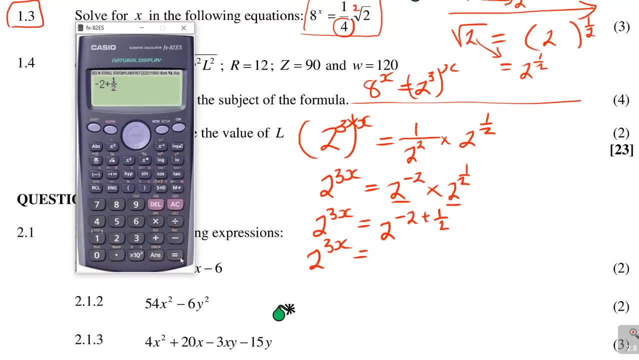 I always try to use My calculator as much as I can To avoid my general knowledge, Because you exhaust your mind. If you try to work mentally, Just rely on the calculator, Because there is a long way to go. Remember, you are in question number one. 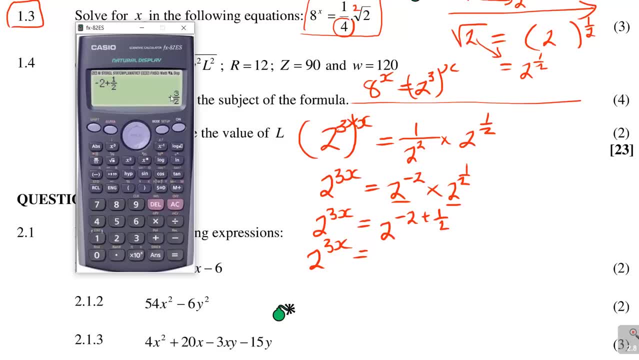 So you don't want to start using your mind To be calculating what is minus half times plus half, Minus 2 plus half. Your mind is thinking. But already you are exhausting your mind. Just punch the calculator, It is still fine. 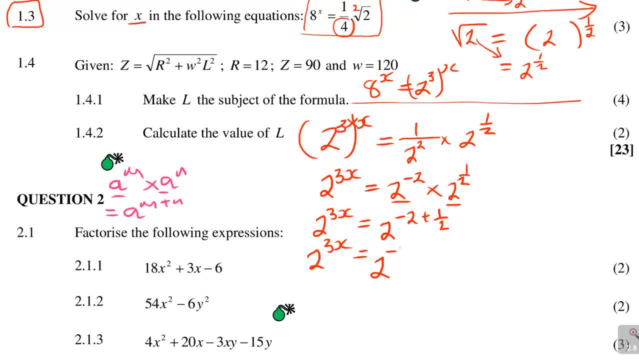 So you see the answer: It is negative 3 over 2.. So it is 2 to the power of negative 3 over 2.. Now an important law here You are going to apply, And the law says When you are given. 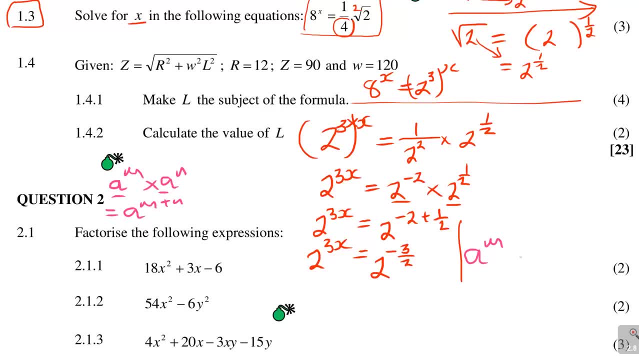 Like this: If you are given a to the power of m Is equal to a to the power of n. If the bases are the same, You also equate the exponents. You put an equal sign. So therefore It means m is equal to n. 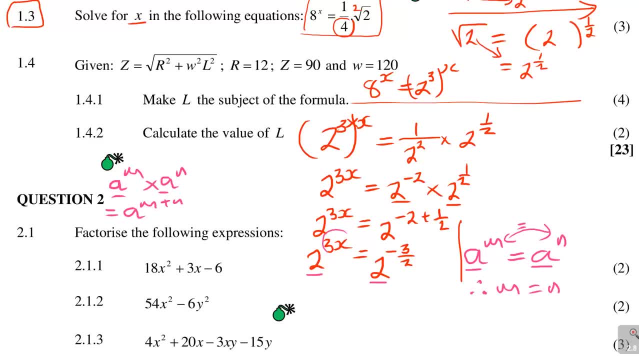 Look at this. The bases are the same. Therefore it means that is equal to that. So how do you write it then? We are going to say: 3x Is equal to minus 3 over 2.. That's what it means. 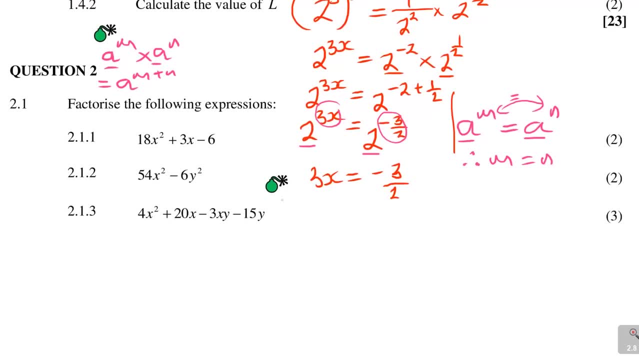 And then the only thing there is simpler: Just solve for x. How do you solve for x? You divide by x, So you can divide by 3.. Again, Just rely on the calculator. x is equal to, But you need to be sensitive how you punch this. 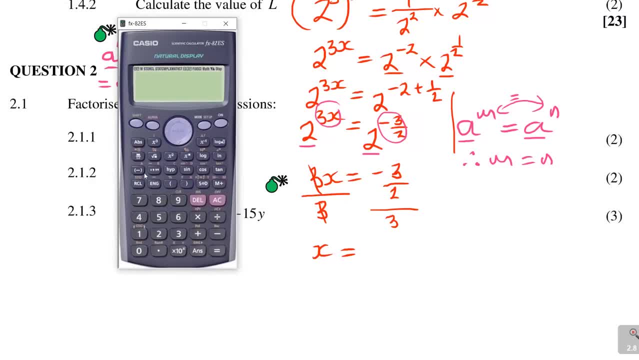 Sometimes students get confused on how they do this. So first thing: first You have that fraction, It's negative. Then you've got that. You see the fraction where it is: It's 3 over 2.. That is on top. 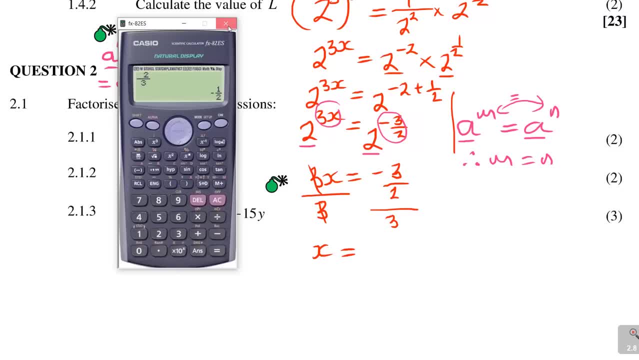 Divided. That is the one that is divided by 3.. Don't do like this. They see 2 division lines. They press, They press. That is fine, But sometimes you need to be careful. I see that the bigger one is at the bottom. 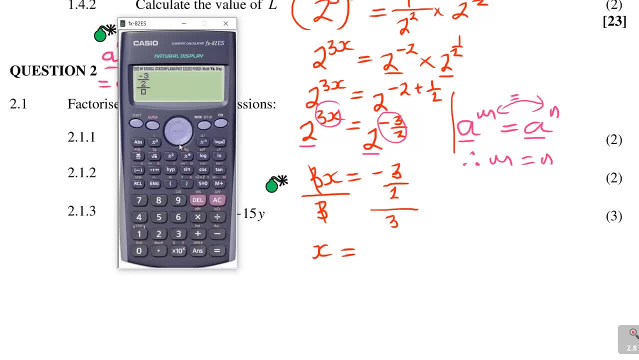 So it will be negative 3 over 2.. This one works well Over 3. It works well. But I will show you some other time Where it is not proper for you to, For example, If I give you and say: 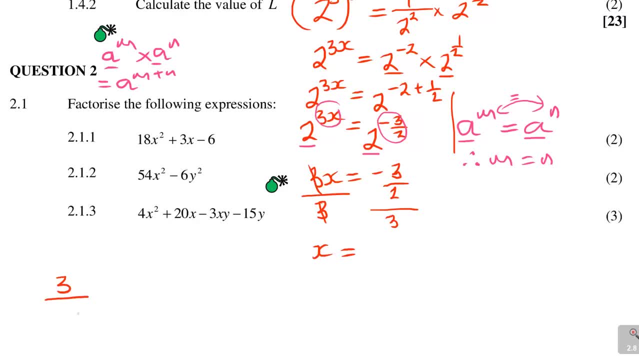 It's 3 over 2 over 3.. You see, the fraction now is opposite. So if you do that now, You are going to get it wrong. Look at this: If you say The way to punch this is 3 over. 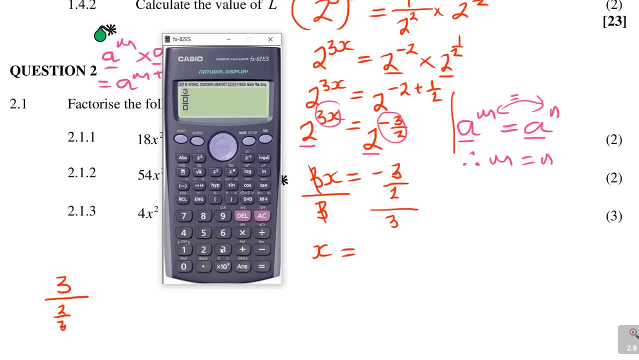 Then at the bottom- That's where I put my fraction- Then I've got 2 over 3.. So you see how it's like That's the right way, It's 9 over 2.. But if you just do this, 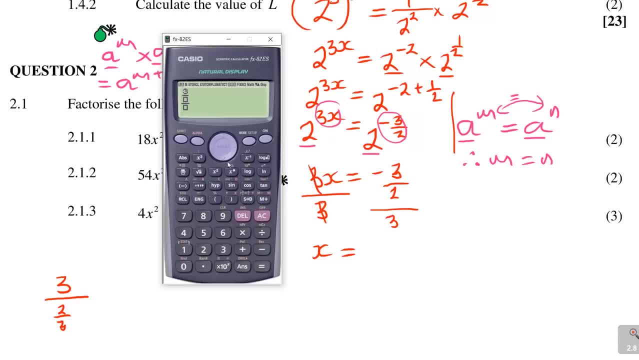 Fraction. You are going to say 3 over 2 over 3.. And then when you do that This time now, You are not going to get it right Because at the end of the day, It's not going to give us C. 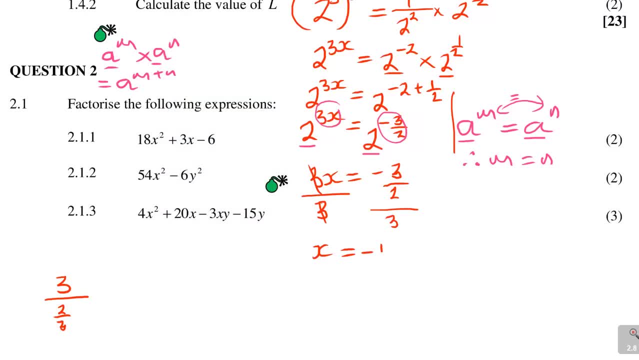 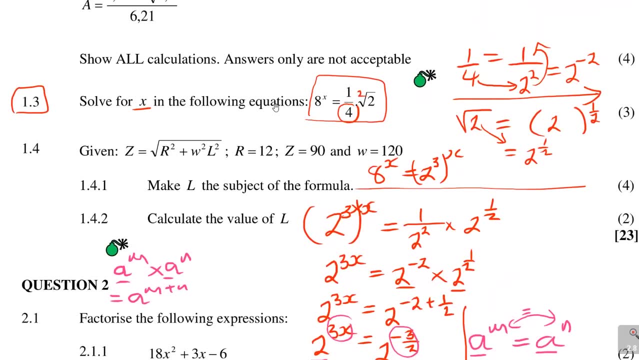 It's now giving us a half, So you need to be careful. The previous answer, if you remember, It was minus 1 over 2.. So if I take that answer here, You definitely need to prove this If I put minus 1 over 2 here. 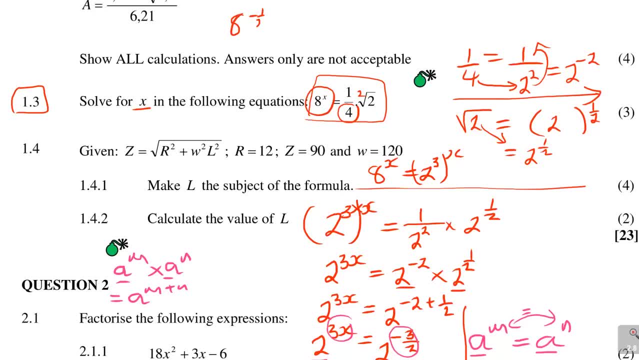 To say what is 8 to the power, Negative 1 over 2.. It must give me this: 1 over 4.. Square root of 2.. So I just need to know My left hand side And I just need to know my right hand side. 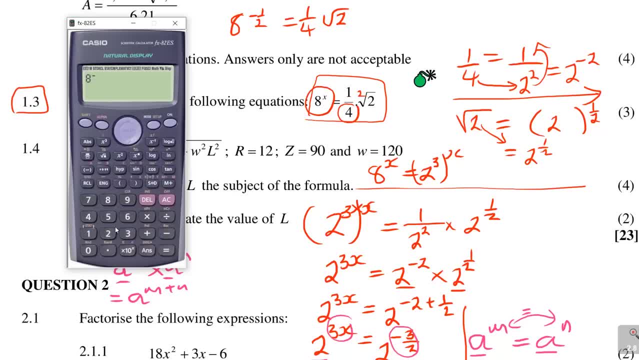 So if I say 8 to the power of Negative 1.. Let me do this To say Negative 1 over 2.. If I do this, I'm getting a funny answer: 0.3535.. Remember this answer. 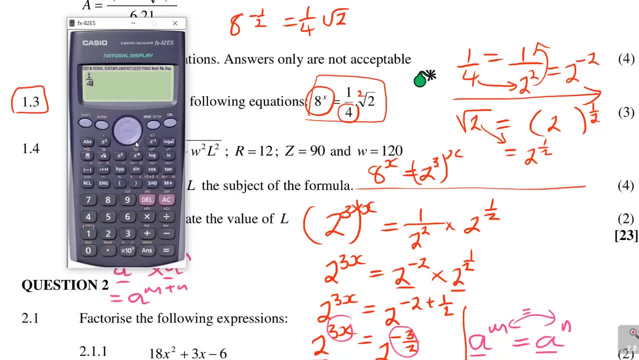 I do also the other side, 1 over 4.. Times Square: root of 2.. It must give me that 0.3535.. 0.3535: you see The left hand side, The right hand side balances. 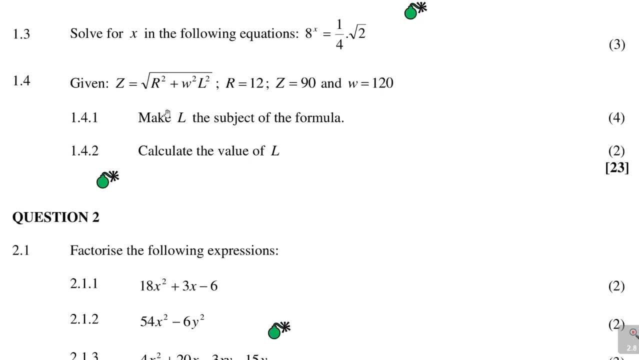 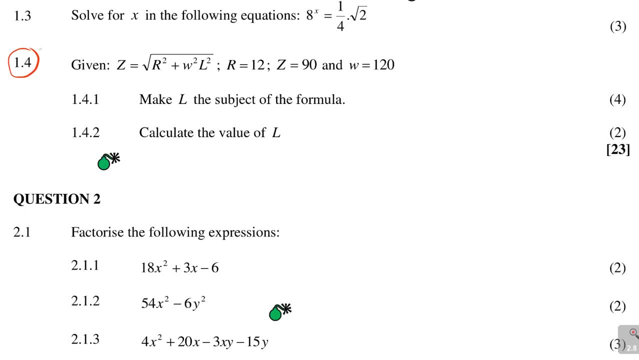 It's correct, guys, Test your answers. You are guaranteed of the 23 marks. Let's finish up with this: 1.4.. And then we call it a day. Remember again to tune in On these coming days Before your final exam. 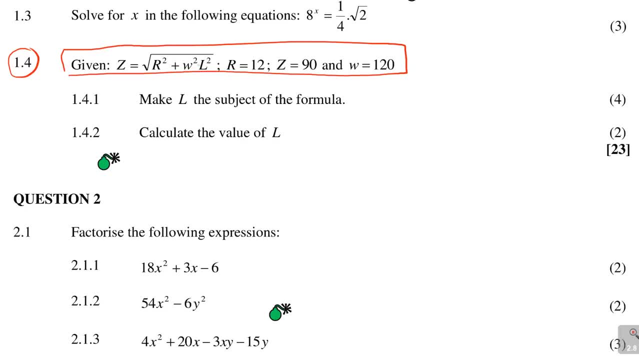 And then this one says: We are given this information, We are given Z is blah, blah blah. We are given the value of R, The value of Z And the value of W. These are common questions. First they will say: Make L the subject of the formula. 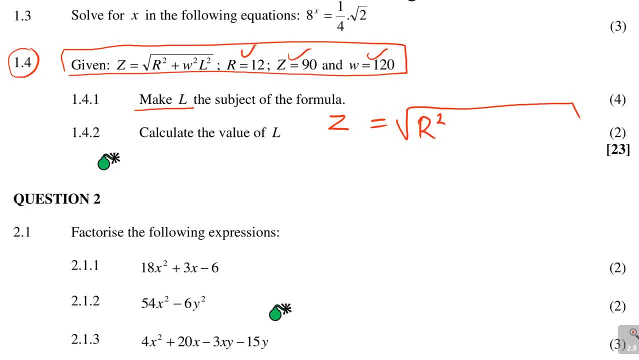 So what you are given is: Z is equal to the American Called Z. So Z is equal to Squared. We call it Z, They call it Z. Let me make L the subject of the formula. First things first, I need to get rid of that square root. 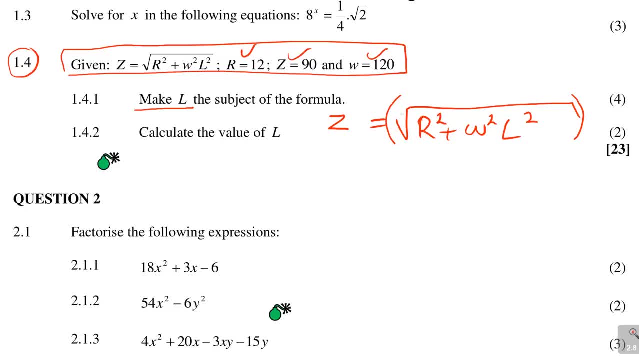 What you do, Put a bracket And to get rid of the square root there, You need to square there. But what you do on the left, You also do on the right. So now it will be: Z squared is equal to. 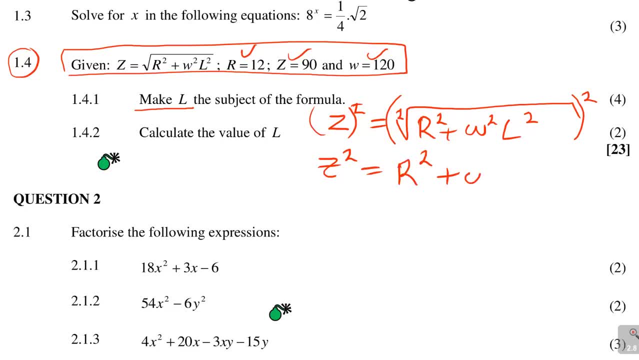 Because of that, The square root is R squared plus W squared, L squared. That's what you just did. The next thing: There is a plus sign here. It means the R can join the Z squared. So Z squared Minus R squared. 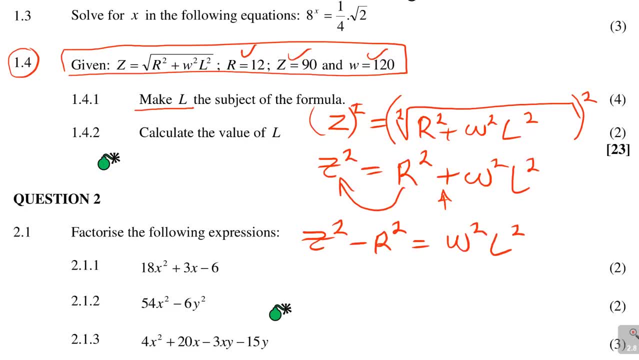 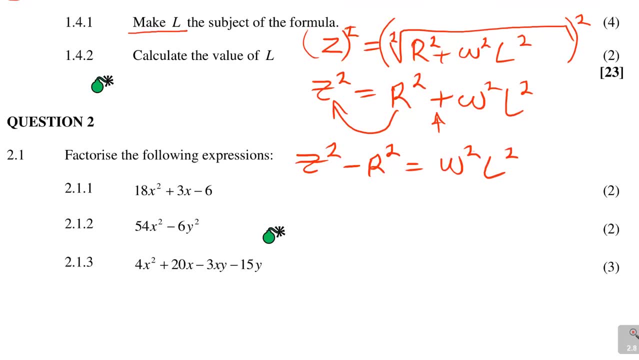 Is equal to W squared, L squared. This is just. I always see this algebra As one of the most important ways Of learning algebra. They are multiplying, And the opposite of multiplication Is division, So which means to get rid of W squared? 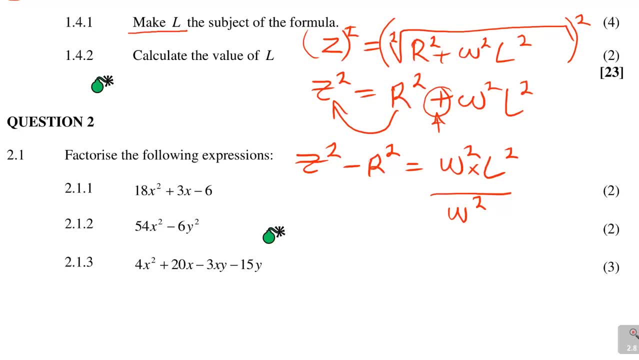 I must divide by W squared Y, Because it was multiplication. Here it was addition. You see, opposite was subtraction. So always remember that. But what you do on the left You also do on the right. Why? So that you can get rid of that. 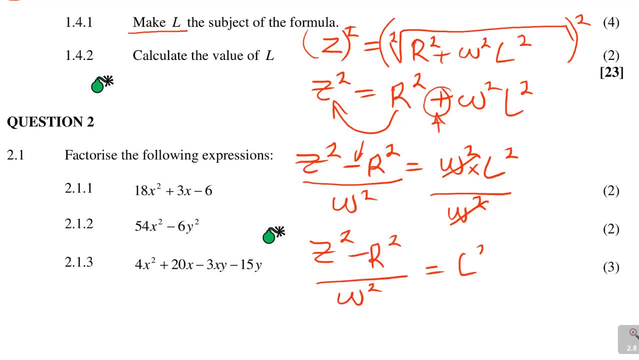 So you have got L squared. The next thing is for me to get rid of the square. To get rid of the square, Remember to get rid of the square root. I squared, But to get rid of the square, Use square root. 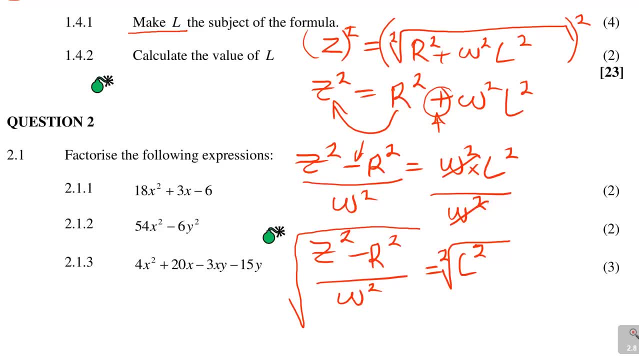 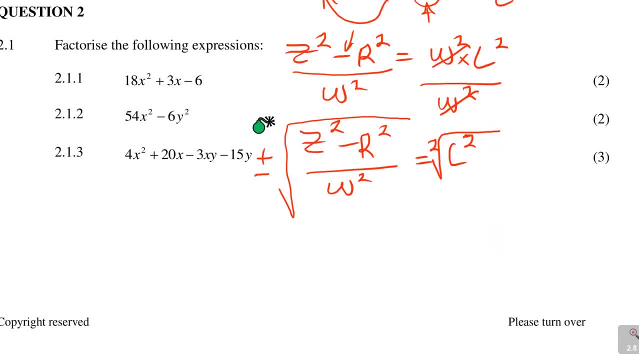 So this is just the opposite. See what I am doing. But what I do on the left, I do on the right. But here you are allowed to say plus or minus. It's a lesson for another day, But you can leave your answer like that to say: 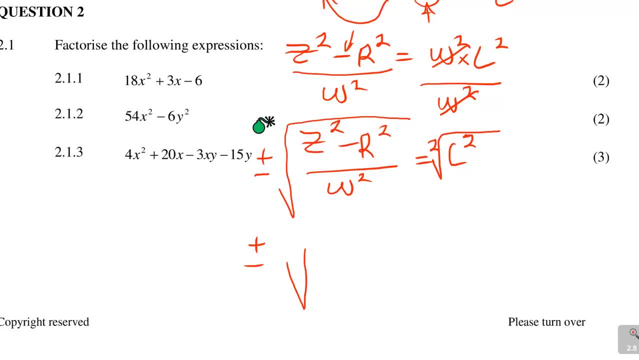 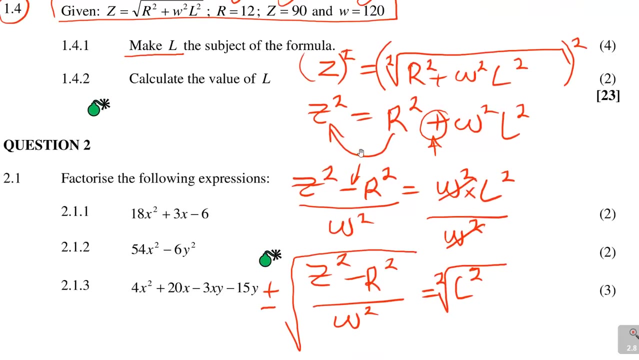 The answer is plus or minus. So what I am going to do Is to get rid of the square root of Z squared Minus R squared Over W squared Is equal to L, And then The question is not done. 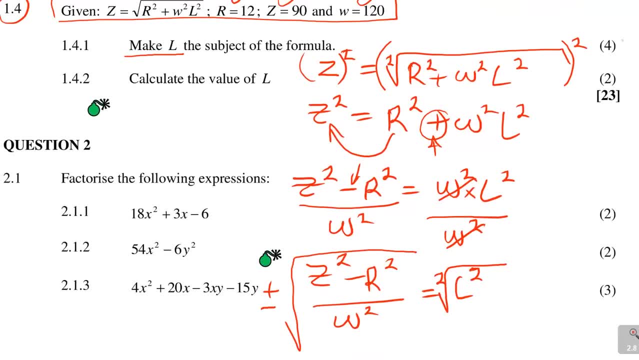 That is how you get your first four marks. So you get the first four marks. Then the last part of it says 1.4.2 says Calculate the value now of L. Remember they gave you some information to say In here. 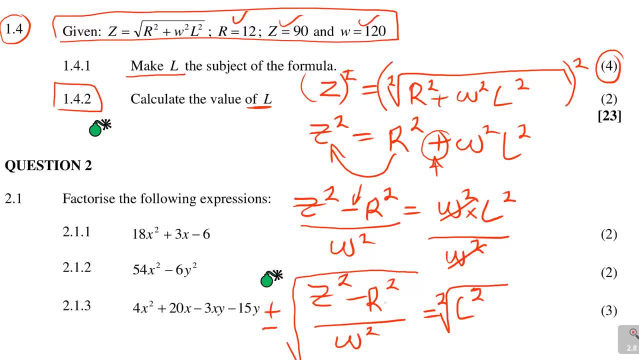 R is 12.. So here you have got 12 squared, And then Z is 90.. There you have got 90 squared, And then W is 120.. So you have got 120 squared. So that is basically what you will be having here. 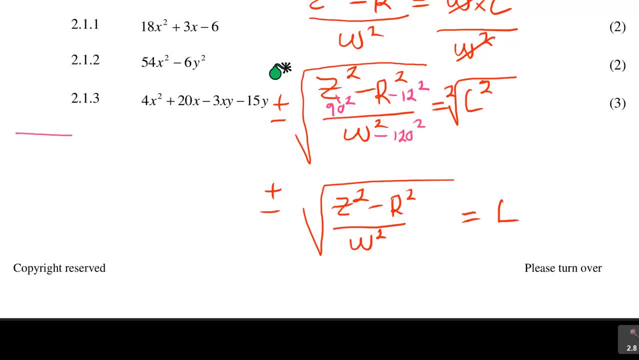 I was just writing it down So that it will be easier for me To follow up. So if I can finalize it, 90 squared- Actually I must write it. This is my. L is equal to 90, squared Is just two marks. 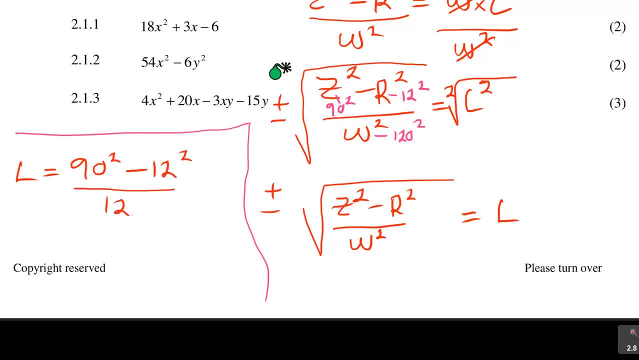 Minus 12 squared Over 120 squared. Don't over think it, Don't start to make it In a way Like long and stuff. Just go straight to your calculator And it will just give you an answer, You understand.